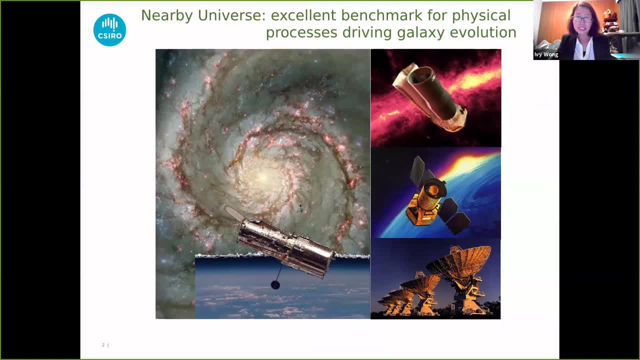 Because with the technologies we've had in the past 10-15 years, we've really been able to not just look at galaxies as a global thing, but rather we can look at nearby galaxies and study the individual or the masses of star forming regions. So here are some of the giant star forming regions within the world, full galaxy, and we've got the HST. that's about to be retired. 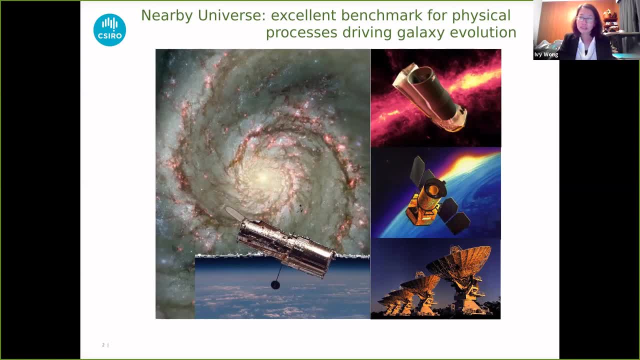 Both Spitzer and GALAX have already retired and we've got our little compact array, SOGIA, here representing the radio, showing all the different perspectives that you can see and probing all the different wavelengths and emissions mechanisms that exist within even a single star forming region. 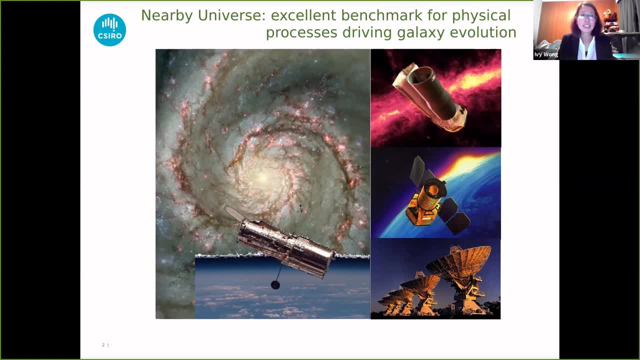 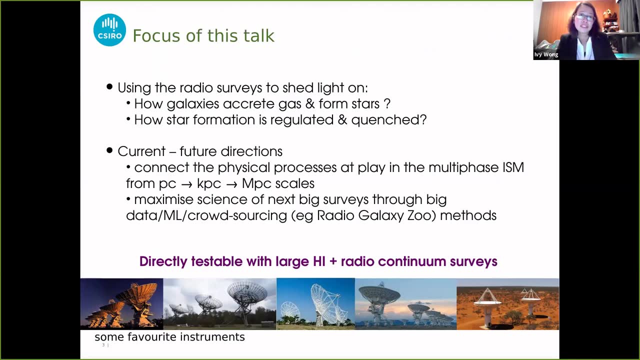 So the focus of this talk really is to to focus on the point that the next generation radio surveys will truly help us understand how galaxies get the gas to form stars and subsequently evolve. And one of the main questions that we'd like to get answered is how star formation is regulated and quenched in galaxies. 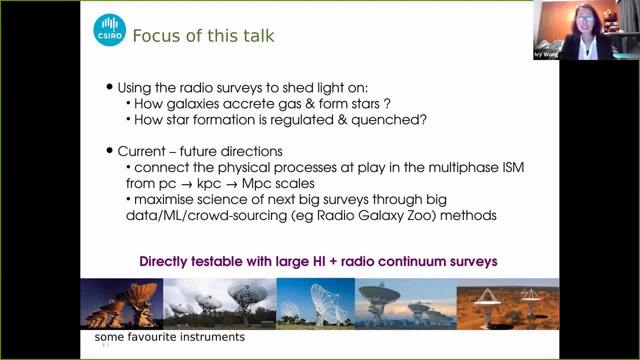 Because we have a rough general idea of how this occurs in galaxies, and we've got a lot of data on this, But in terms of the actual physical processes at play, we still don't have this in fine detail or any detail just yet, And so it is my personal prediction that from now to the next 10 or 20 years, the main game is to connect the physical processes we know. 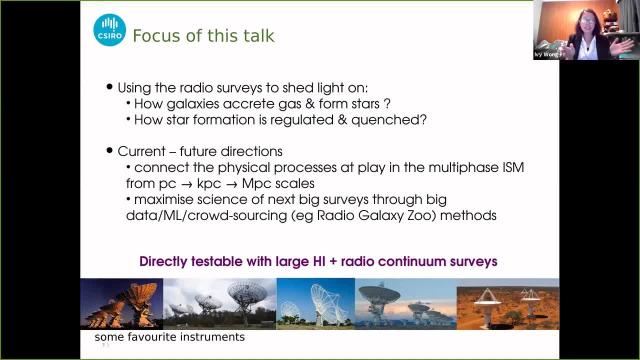 occur in the multi-phase interstellar medium, from the Parsec scales to the kiloparsec scales, out to the megaparsec scales, And what we'll need are the new instruments that are up and coming, but the problem is, these new instruments introduce a huge amount of data, a huge volume, and so it will require. 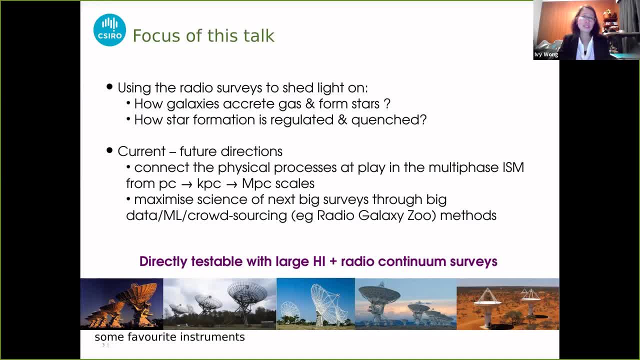 less traditional methods and more alternative methods in order to maximize the science output from these particular next generation surveys. And much of the science that we're hoping to shed light on are quite directly testable with the next generation large H1, which are atomic hydrogen. 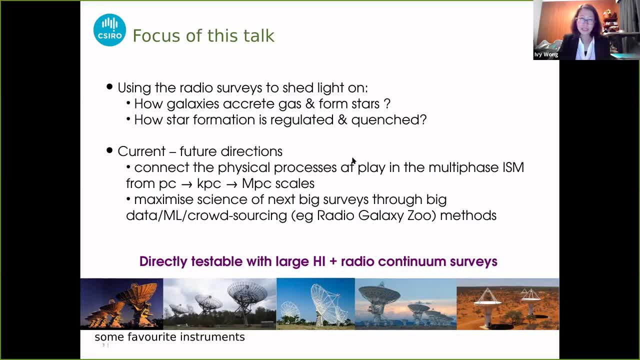 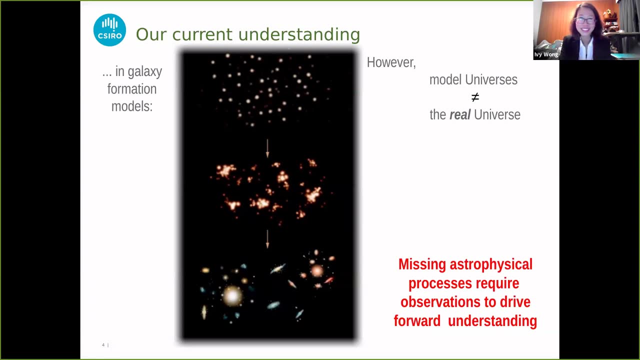 or the radio continuum surveys, and here's a quick collage of some some of the instruments whose data you possibly see in this particular talk. So how do galaxies form? I know that this particular astral department is not really focusing too much on galaxy evolution, but in a 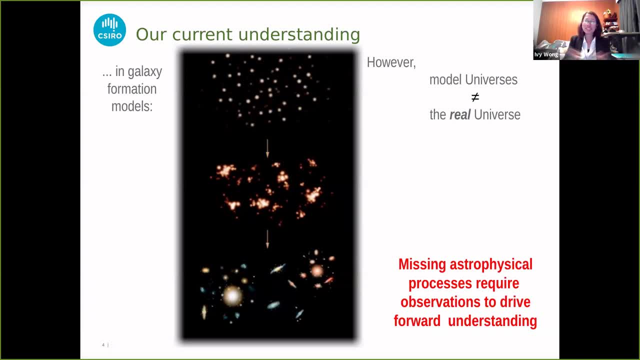 very small nutshell. we assume that you've got the beginning of the universe at big bang, and then, after recombination and reionization, you've got baryons painted on at sufficient densities, and then we see the stars and galaxies as we see today, and so these are our cosmological 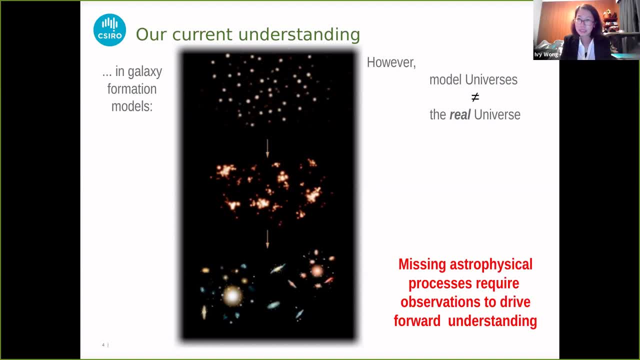 simulations that have been evolved through 13.7 billion years Now. unfortunately, what we observe and what comes out of these models are not quite one and the same, and so what this suggests is that we're missing quite a few of the astrophysical processes that I play. 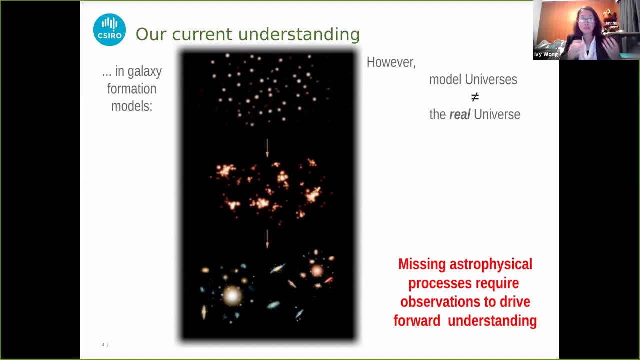 during my talk. So I'm going to show you a few of the astrophysical processes that I play during galaxy evolution, and this is the missing bits of the puzzles that we're trying to solve with observations. In fact, these are the observations are the only way you could constrain the. 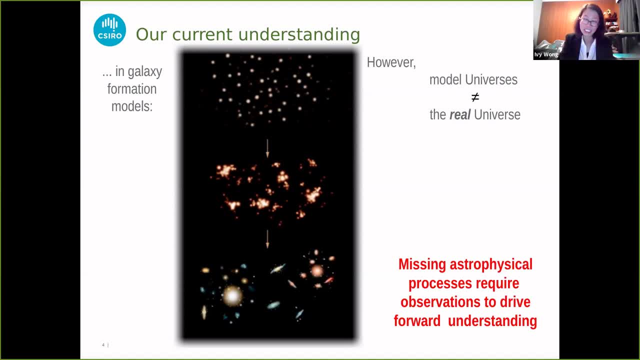 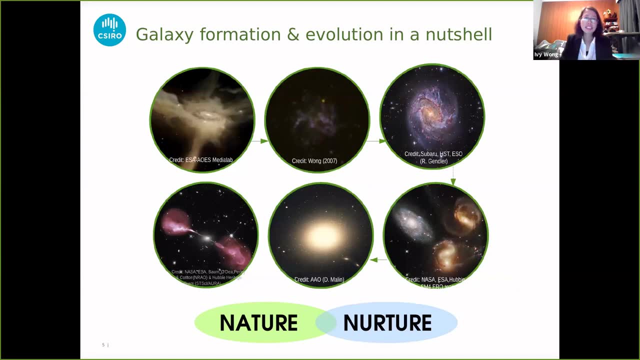 number of processes or number of things that could happen during galaxy evolution, And here's galaxy evolution in a nutshell. So the galaxy has to create some form of pristine gas. so typically there's atomic hydrogen from which molecular gas will form, and subsequently stars, and over time such a galaxy would evolve into this. 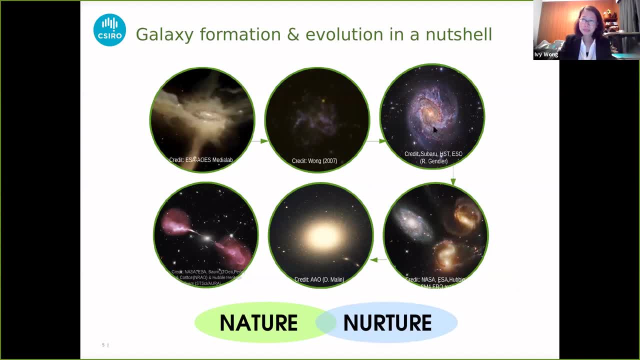 neat little m83 spiral you see here in the third bubble. and if the galaxy lives in a closed environment with other galaxies, interactions- tidal interactions and other forms of interactions, such as ram pressure- will distort or affect the way such galaxies will evolve. and finally, after all the interactions have occurred, the galaxy will be able to evolve in a closed environment with other. 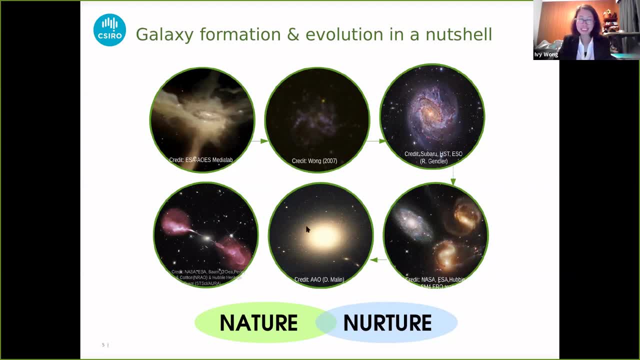 galaxies interactions, tidal interactions and other forms of interactions such as ram pressure, will distort or affect the way between different. you know, combining the angular momentums and of different galaxies coming together, interacting, will get somehow such elliptical, spheroidal beasts that you see here Now what I don't actually put in this picture. 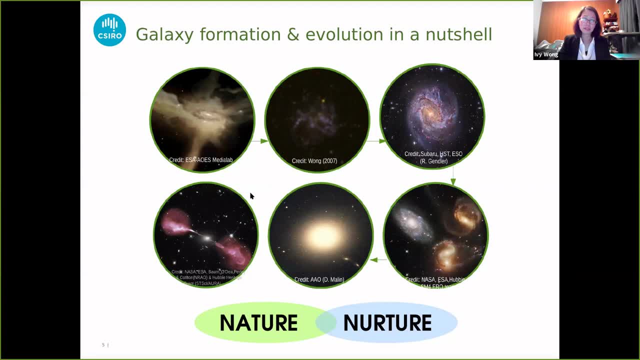 is how galaxies grow their central supermassive black hole. so this little cartoon bubble here shows you the Hercules A galaxy. It's a spheroidal that looks roughly like the passive galaxy here. It's a spheroidal that looks roughly like the passive galaxy here. 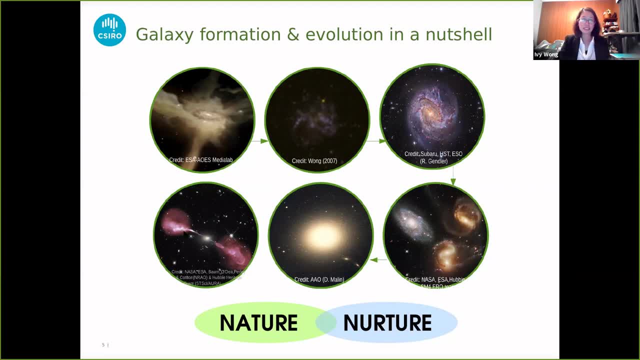 It's a spheroidal that looks roughly like the passive galaxy here, But it's creating gas and ejecting huge amounts of radio emission, shown in the purple, and as the galaxies grow, it also grows its central black hole. however, we we do not know how this feeds back in terms of energy feedback onto the. 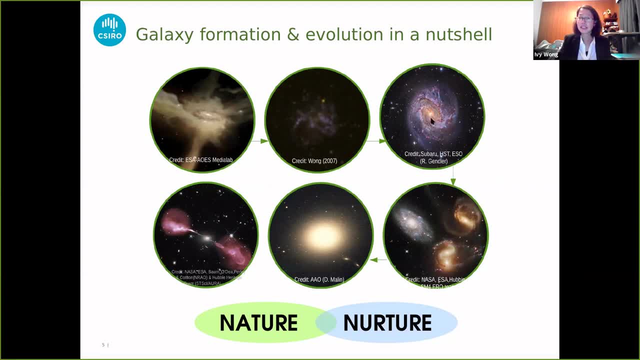 galaxy. we've got a lot of models, but actual direct evidence of how growing its central black hole, as well as star formation. the core evolution of this is not a very clear picture at this point, and so these are some of the. this is one of the main hot topics that galaxy evolution astronomers 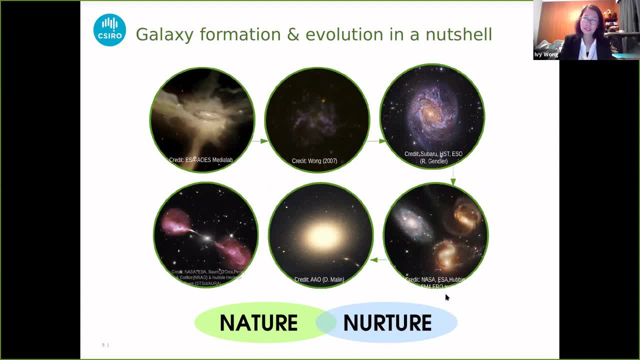 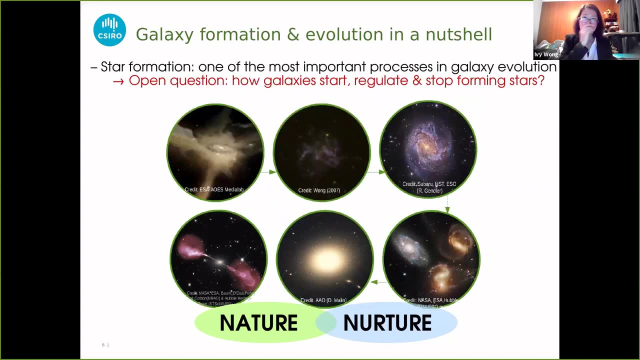 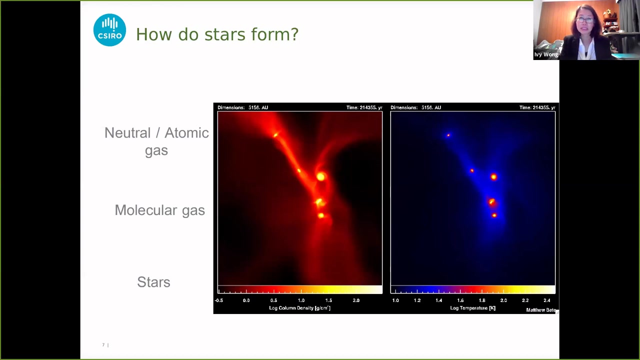 are currently working on. so, as with everything in in nature in our world, we've got nature versus nurture, so let's see. so yep, the open questions are how galaxies start and regulate and stop forming stars. so how do stars actually form? once again, i'll paint you the very general picture. 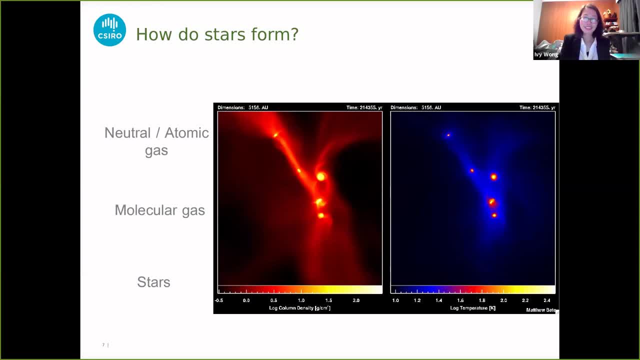 that, you know, semi-analytic modelings will tell us and what we know in general happens, which is that we start off with some atomic gas that forms the initial reservoir from which molecular gas and stars will subsequently form from. so here's an illustration from a model by Matthew Bate and Exeter. 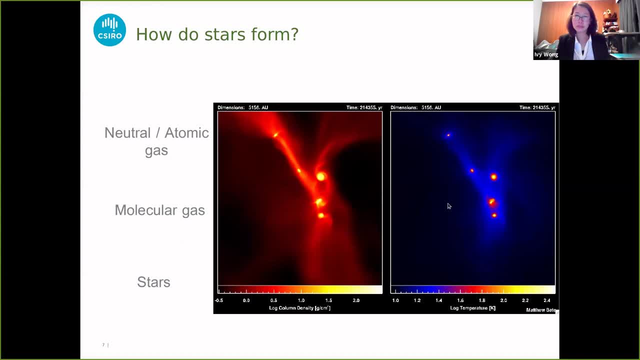 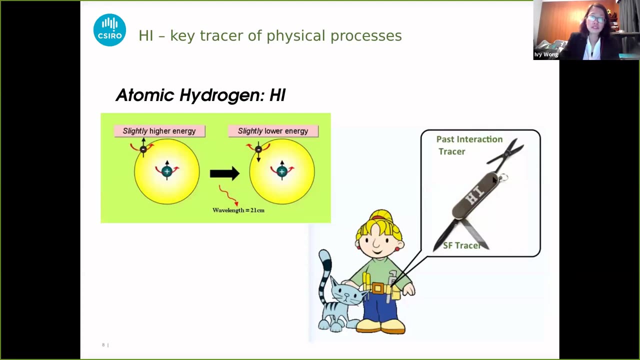 and the left shows you the density of the gas and the right shows you the temperature, and so you can see that gas comes together and, at sufficient density, stars form where the bright coals are. now, where does atomic hydrogen come in? what? why is it important? so, hopefully, by the end. 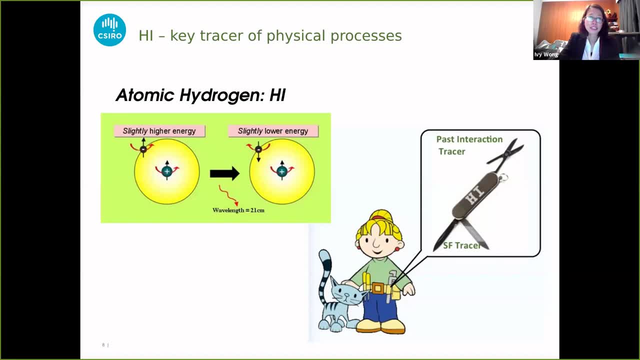 of this talk, you'll be convinced that H1, an atomic hydrogen, is a very important tracer and much quite a useful tracer for past interactions as well as a good tracer for the particular process. so let's see what we've got here. so we've got a little multi-tool kit. 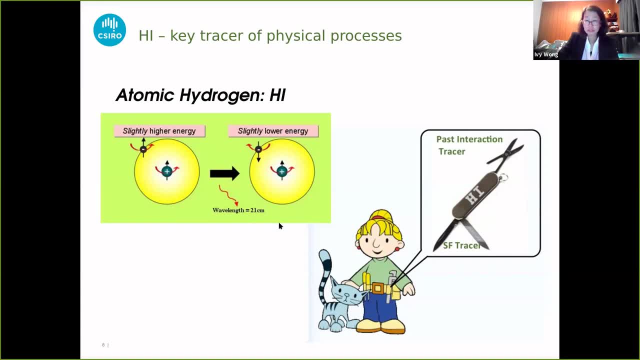 and so we've got a little multi-tool kit, and so we've got a little multi-tool kit, and so we've got a little multi-tool kit. how we observe it is through this 21 centimeter 1.4 gigahertz frequency, and we get this emission through the hyperfine transition, for when the 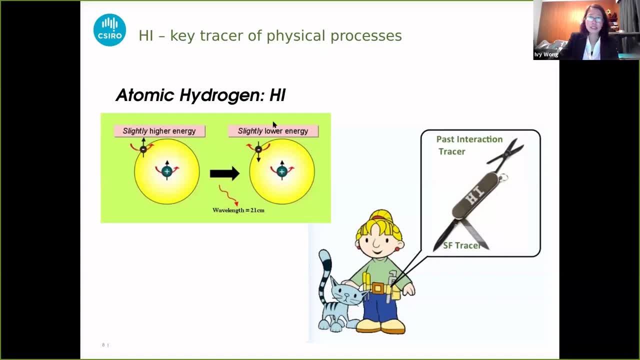 electron spin spins back down from a higher state to a lower state and so as we move out we get potentially, with the sk low. we could see the H1 at the epoch of reorganization potentially. but bring it, bring it back to what I actually work on, back to the nearby galaxies. 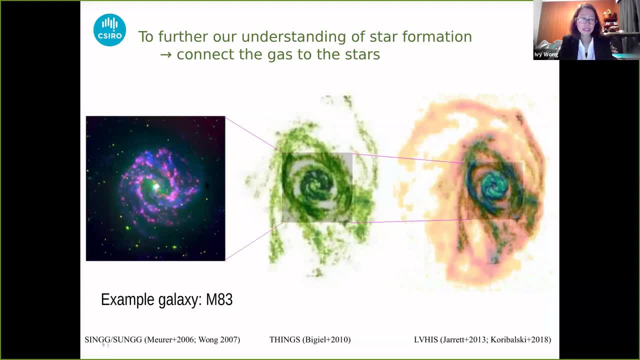 here's an example of M83. what we have here is the R band in green, the blue gives you the ultraviolet, far ultraviolet, and the pink is H alpha. and so what we're showing here are the two general, two populations of young stars traced by the H alpha and the UV, the older stellar population in that. 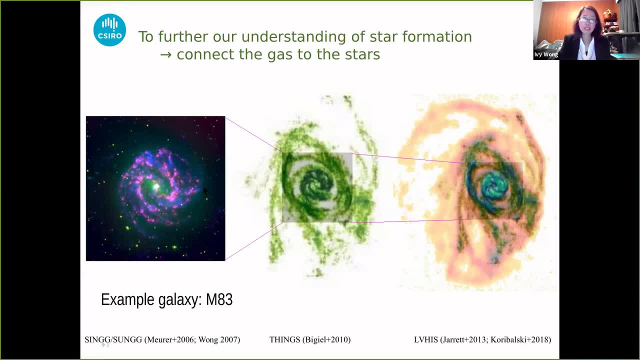 green fuzz that you see there, and when we look at this particular galaxy in H1, you can see how much bigger the H1 reservoir is and how the spiral arms actually extend much further in in H1 gas than it does in the stellar content that we see. in fact, if you were to look at this, 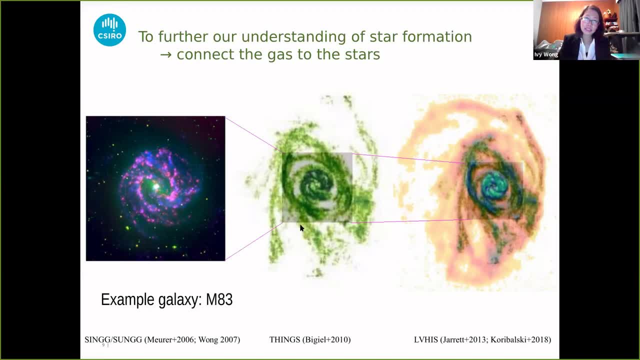 galaxy. quite closely in the UV you'll see extended UV arms following the structure of the gas, and if you zoom out even further you can see how much larger it keeps getting so through the different H1 surveys. so the reason why I'm showing you both the things- H1 survey and the Elvis H1 survey- is that part of how we observe H1. 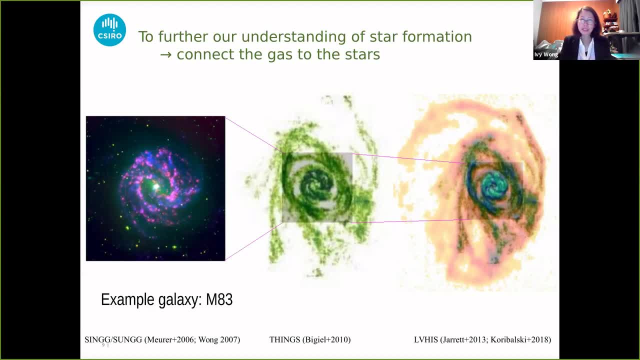 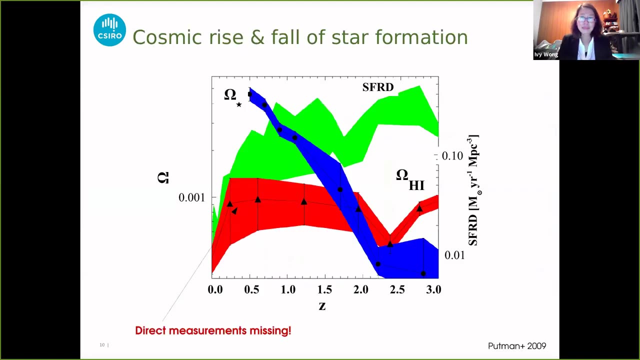 or how we observe radio observations is through interferometers and depending on your array configuration and sensitivity, you probe the gas at different densities and angular scale. so it's good to have all the various angular scales so you get the full picture now in the universe. here's a. 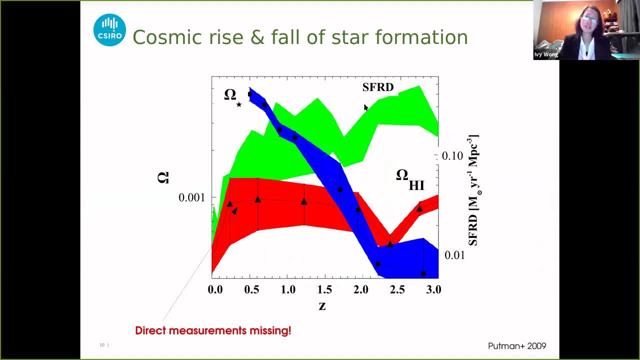 cosmic density diagram. we know that since redshift of two, the star formation rate density has plummeted by over, you know, several factors of tens. so what's going on, see we? we understand basically the stellar density and the star formation rate density, but the constraints on the 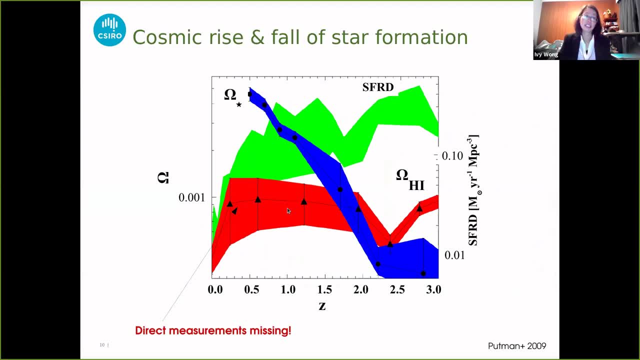 the H1 density is actually quite sketchy, and the reason why I say it's sketchy is because huge surveys in H1 have only gotten out to about redshift of zero all these data points. so, Evie, I wonder. I mean I wonder if this blue red band are just average of one galaxy or this. 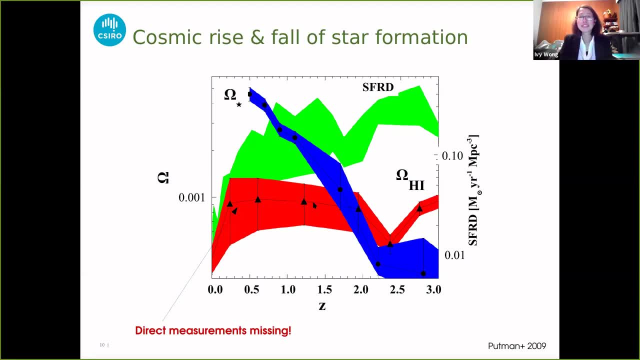 is average. so what I'm trying to say is the neutral gas density is estimated from uh, HST- optical spectroscopy of magnesium, so that it's an inferred atomic gas density of H1 from another tracer, so it's not through direct observations of H1 emission. 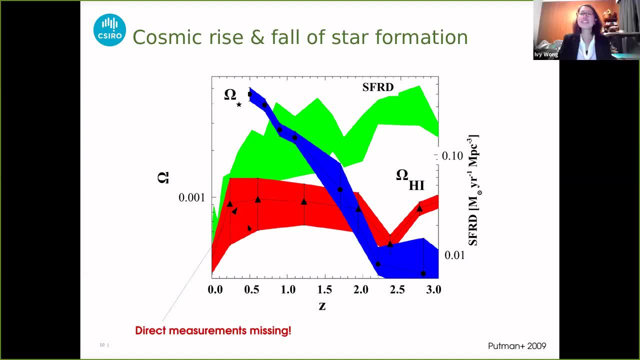 okay, okay, thanks, clear, clear. so this: this is why we're so excited about extending. so the, the meerkat surveys, the ASCAP surveys, I think wallaby will get out to 0.2 if we're not completely flooded out by rfi. so realistically we should get out to about 0.1. 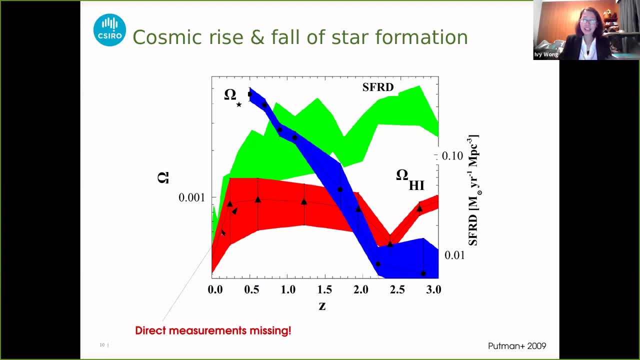 so you can imagine how, how advanced your instrument has to be, how much collecting area, how much sensitivity. you need to actually go further, because as you go further in frequency, what this means is you're going down to lower frequencies. so when you're going down to when one 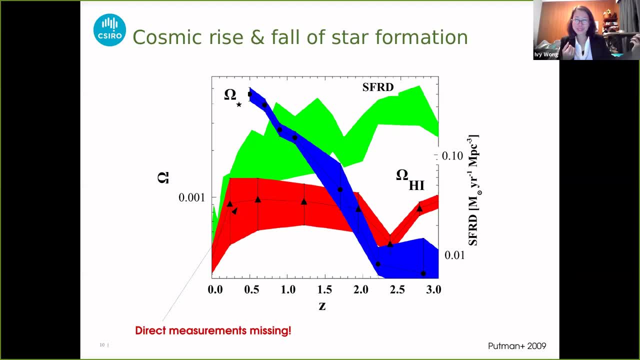 is going down to lower frequencies. you'd like your baselines to be greater so that you maintain your angular resolution, but this means you have to fill up your uv plane by having more collecting area. so one is constantly chasing the sensitivity gain with an interferometer. so, but you know, with the 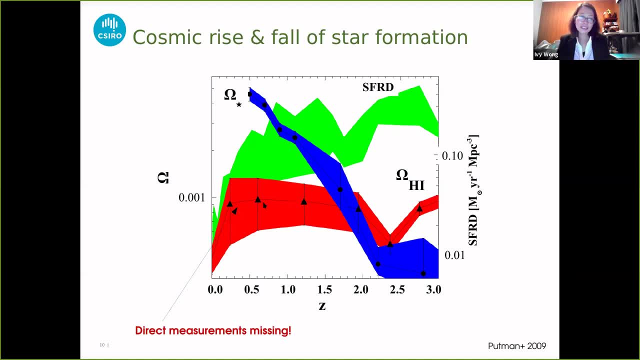 next generation. meerkat surveys and ASCAP surveys. I think my th1 should be able to get out into the 0.5 regime quite easily in a leducative way. I think we're going to be able to get out into the 0.5 regime quite easily in a leducative way. 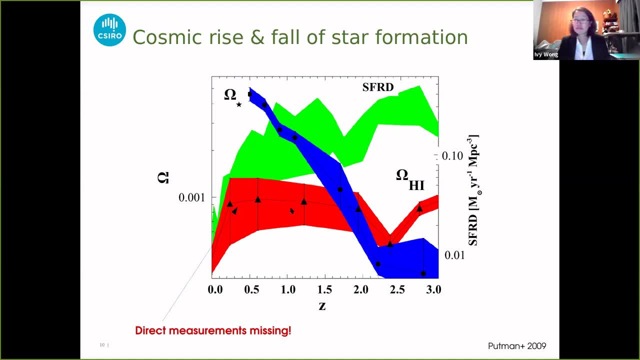 I think we're going to be able to get out into the 0.5 regime quite easily in a leducative way, and the doom is aiming for one. so I see no reason for why there wouldn't be data points out here that would be direct measurements of h1 emissions. so 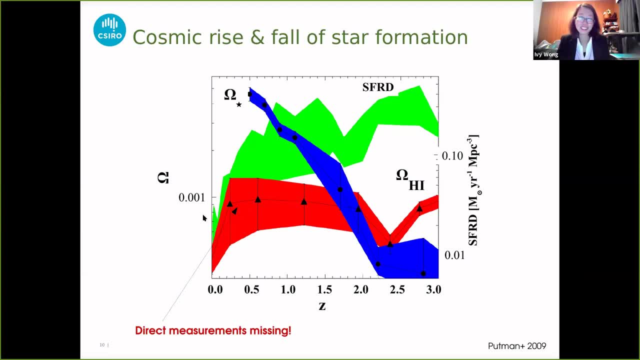 in the next five years. it's a very interesting time for us to watch the space because we will be putting data points out here and, as you see, this is. this plot was from a 2009 mary putnam white paper that was written for the us community, so this is quite an. 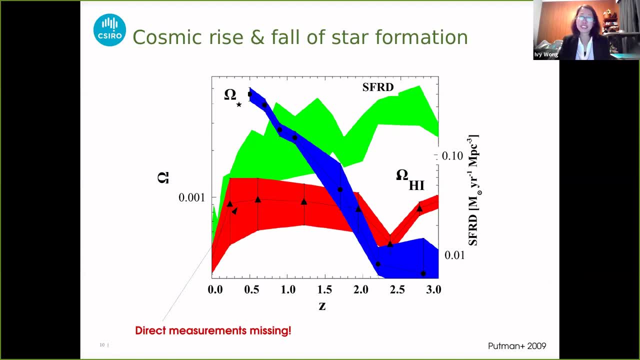 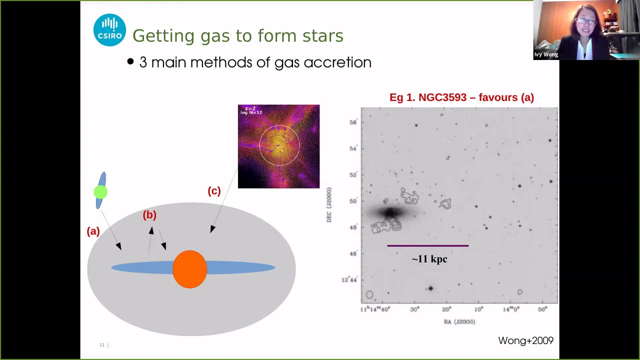 old plot, but the reason I show it is because it shows very clearly how little we understand of the h1 density in the universe since the last 10, 12 billion years. so how do galaxies get gas to form stars? there are three main ways. a galaxy can just usurp gas from a nearby dwarf neighbor. 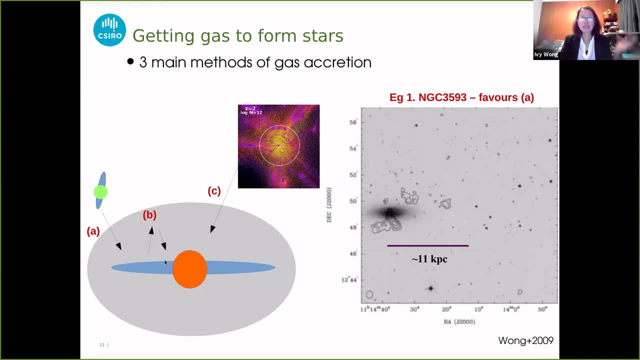 as a galaxy forms stars, the winds blow out the gas and into the halo and then it rains back down through the fountain process, so it gets its own gas that it's expelled back. alternatively, it could get gas at higher ridges from the cosmic filaments and, but typically what we see in the local. 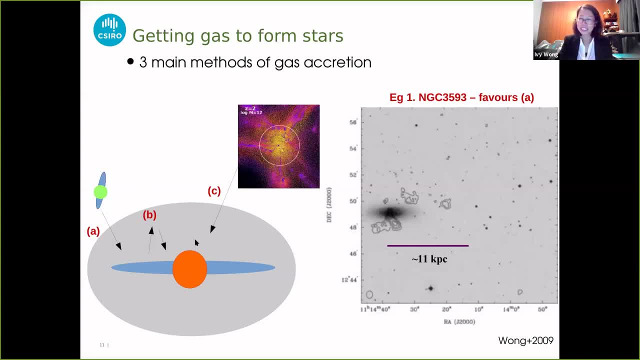 low ridge of universe is case a and possibly case b. here's just an example of some interaction of a counter rotating. so the gas in this case counter rotates with the parent galaxy and if one follows the story of this particular galaxy, it's an interaction scenario. we have also been looking. 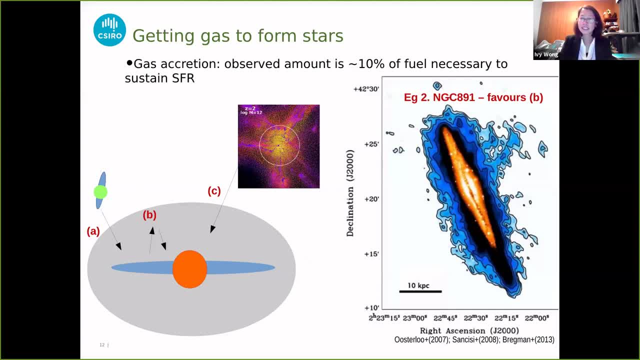 at quite a few galaxies through surveys like halo gas to observe how thick the halo h1 halo could be, and today this is still one of the most popular examples of potential fountain or interaction processes happening to puff up the disk. so but what? what's really, really crucial? 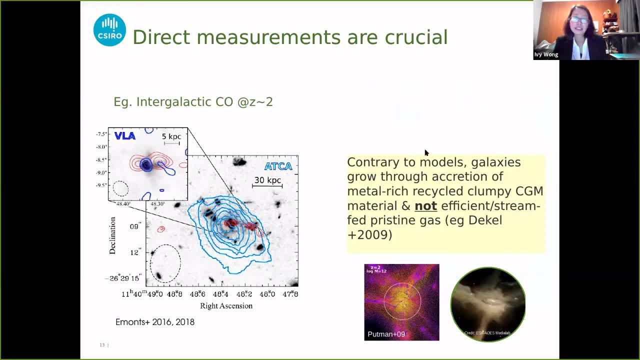 is direct measurements, and here actually i don't use an h1 example, but what we understand of co at very, very low regis seal are very, very compact structures that are restricted to the disk of the galaxy. we don't actually see intergalactic co very much, but here is direct evidence that. 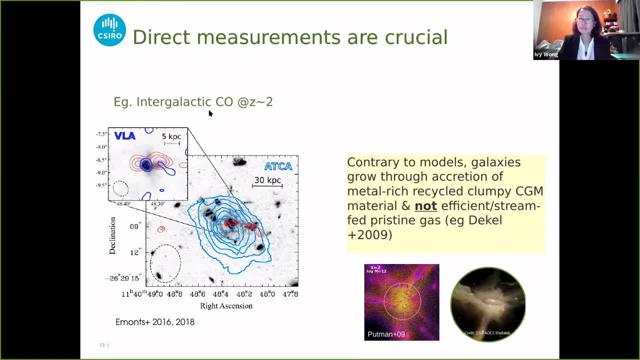 at redshift of two intergalactic co exists, and so this is why direct measurements are so crucial for furthering our actual understanding in that omega H1 regime in cosmology. So- and this is interesting because this shows that galaxies can actually accrete metal-rich- 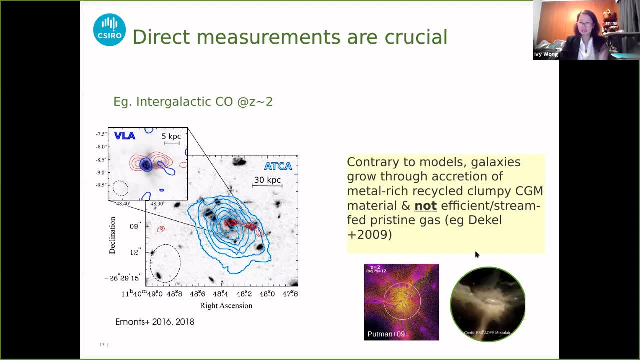 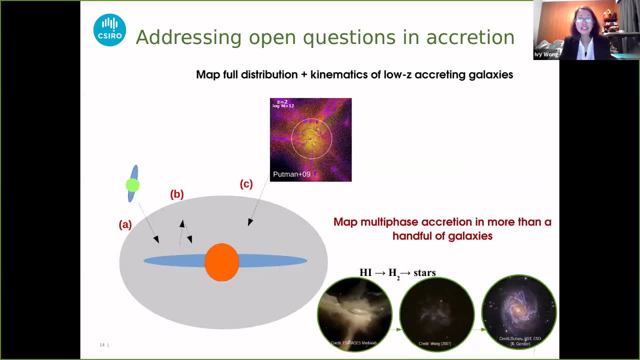 material, not just pristine gas, as was theorized in simulation models 10 years ago, roughly. So, in terms of addressing the open questions in accretion, we really should. one would like to map the full distribution and kinematics of low-rich. 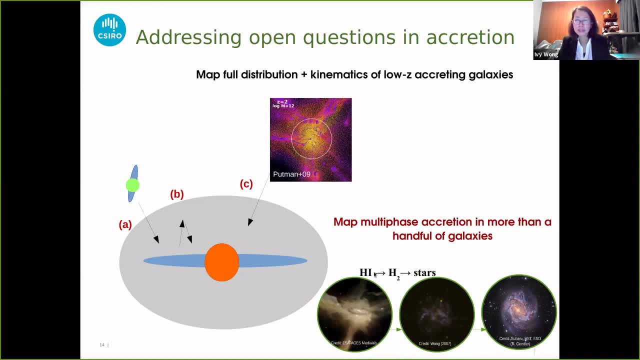 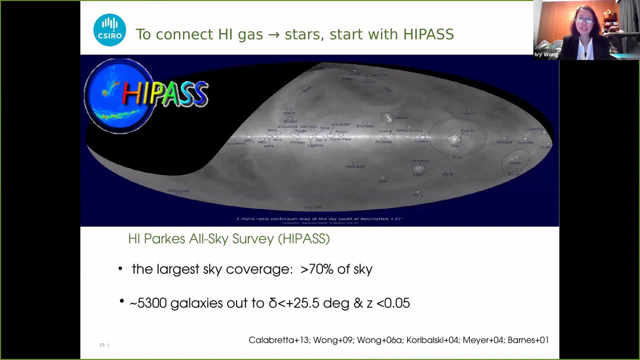 accretion galaxies, so that we're able to track how they convert the atomic to the molecular back to the stars, and how galaxies eventually grow. And of course we've tried doing this. Here's a fairly old survey now: HyPAS. 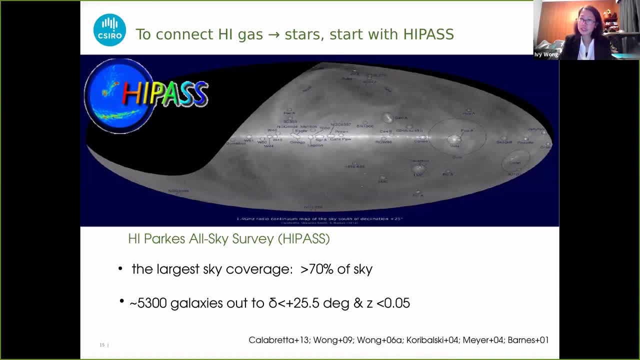 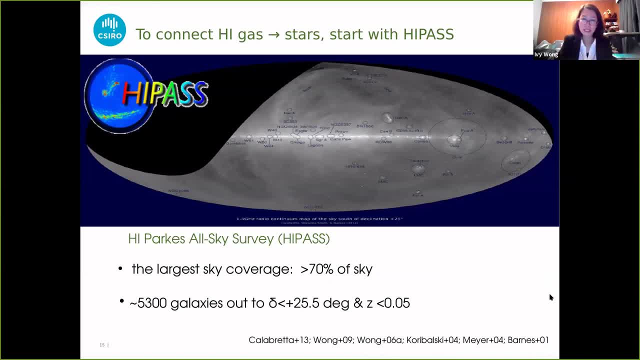 in the state of Australia And basically it's just observed the entire sky it could see. So this observes the entire southern half up to a declination of about plus 25 and a half. It should go out to 0.05, but on average it reaches about 0.01. in reality, sampled about 5,300. 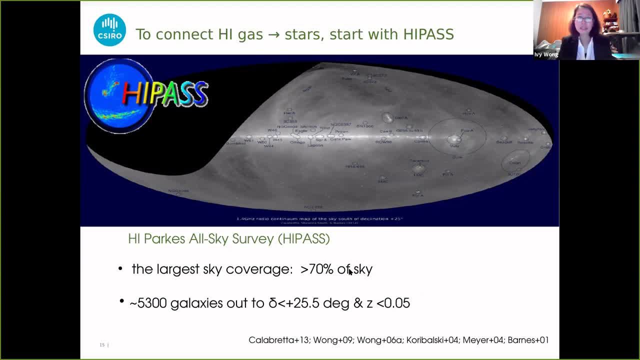 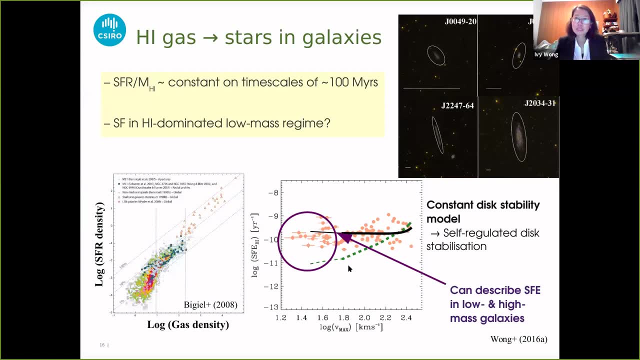 galaxies and lots of papers, But from this, what we could do is to sample galaxies by its H1 mass. The H1 mass is a single mass, and so what you see here is an example of the five orders of H1 mass bin. 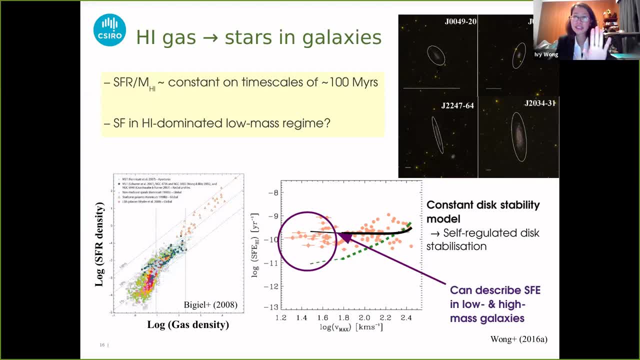 randomly selected galaxies So you could see if they were all put on the same scale, roughly You could see they're not on the same scale because this is the one arc minute bar, so it's a lot smaller and, oops, a lot smaller in some images than others. 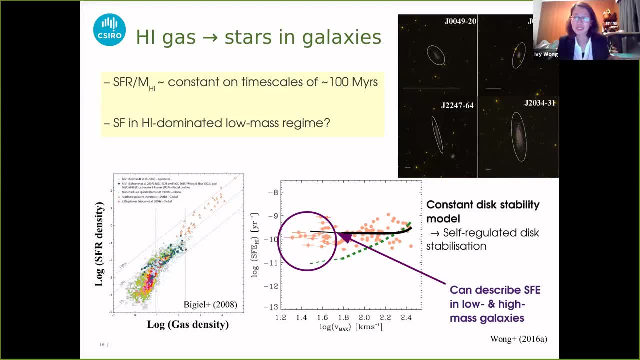 stellar mass. So to study how these galaxies were forming stars, we just selected four galaxies with gas, with the potential to form stars, And what's really cool that we find is that the star formation efficiency, or the star formation rate divided by the H1 mass, is nearly constant on and 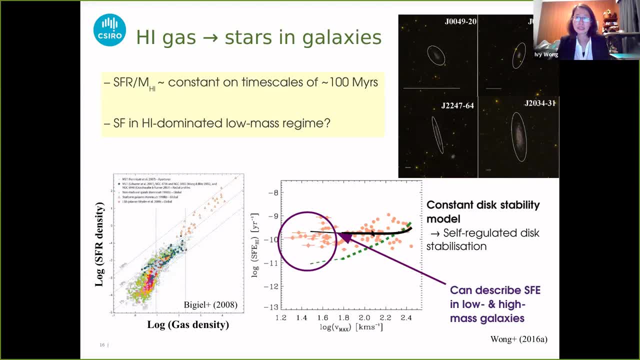 at timescales or on timescales over 100 mega years. So the orange points that you see here are all just observed data points from what we know these galaxies to be. Now this is kind of unexpected because we we know that you know atomic gas. 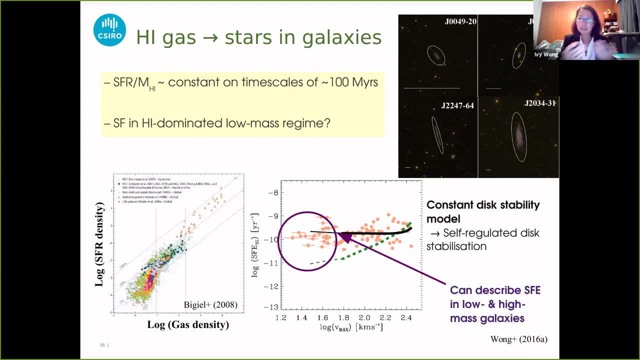 doesn't form stars directly. it goes from atomic gas to molecular gas, then to stars, And the amount of molecular gas between galaxies are different, And the atomic to molecular gas within galaxies also quite different. And so what's going on here? Why? 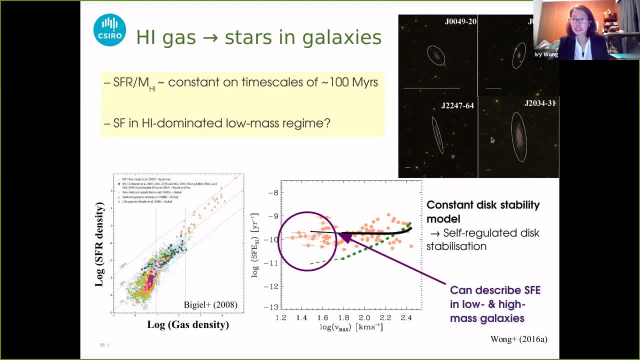 Why is it so constant for all these galaxies across five orders of stellar mass magnitudes? So we had to come up with. well, we didn't have to, but we thought we'll test out a model where we have a constant distability across two fluids, to see if we 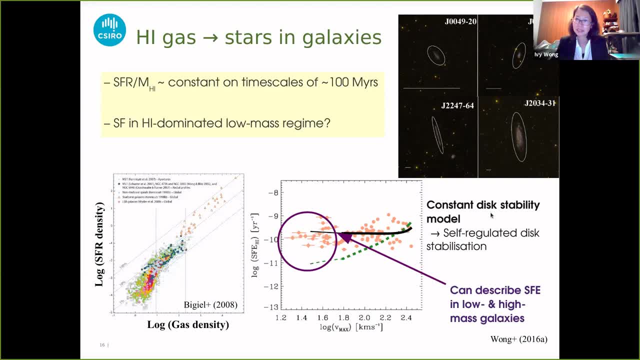 could describe such star formation efficiency behavior across all the various, you know the the huge diversity of galaxies that could form stars. And this is interesting because we know from the Kennecott-Schmidt law which connects the gas density. So this is both atomic and molecular. 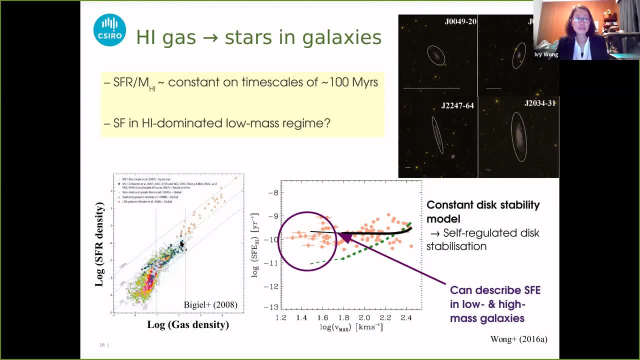 gas to the star formation rate density. We know that for regular galaxies they follow a nice correlation. There's a bit of a. there appears to be a- oops, I have to stop clicking my mouse, Apologies. So there appears to be a jump at the starburst. 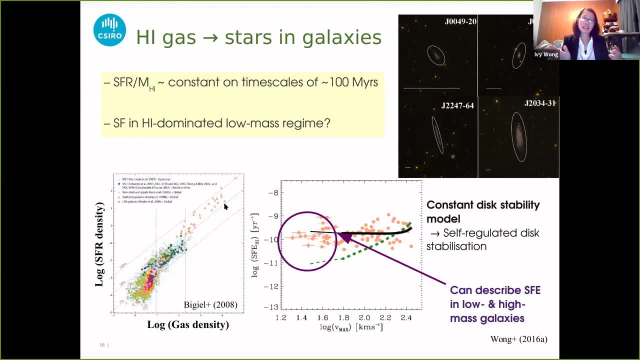 regime. but really we now understand that to be a volume correction And so if we correct it for the actual observed volume instead of a surface density, we convert that to a volume. this would be a nice correlation, But what's still not really understood is this: H1. 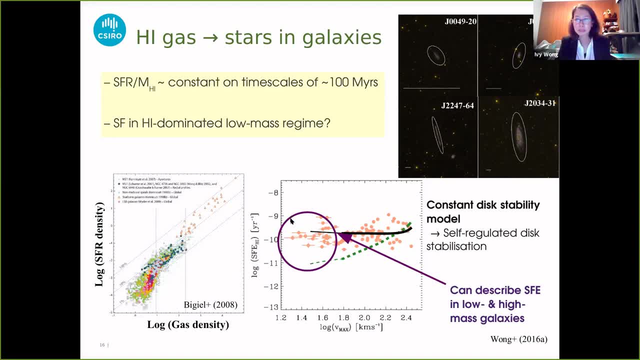 dominated regime. And so what's nice about this particular way of selecting for star forming galaxies is that we we are able to show that actually star formation across all the galaxy is capable. forming stars appear to have a very, very simple, simple star formation efficiency, explained by a self regulated 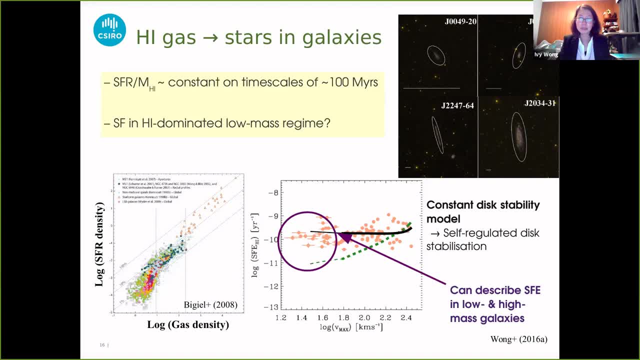 this, this stability parameter. So what is this And why have I shown you this green dotted line that fails? So the green dotted line fails because this is the model, assuming that you're governed by the disk pressure prescribed by your stellar density. So, as you, 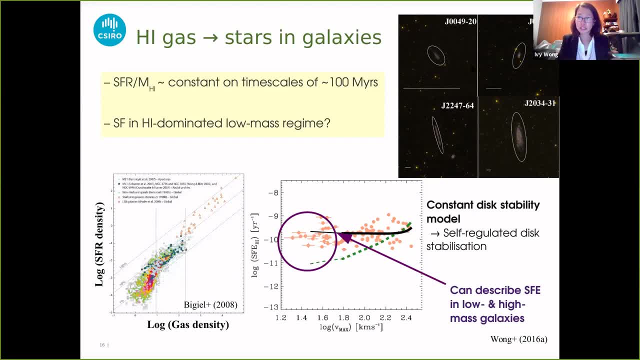 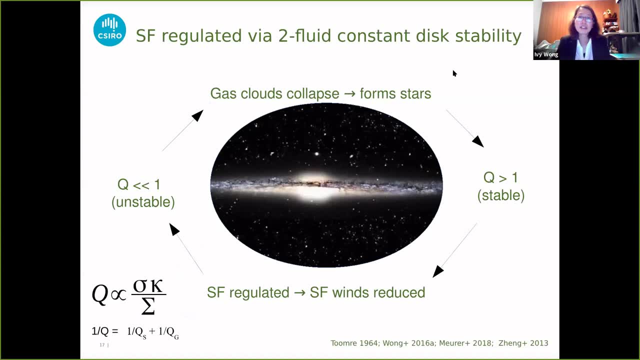 can see from our sample some galaxies a lot more flocculent and fluffier and not, you know, fairly low surface brightness. And so how this stability model works is that it assumes that your constant stability is a constant across your gas and your star. So 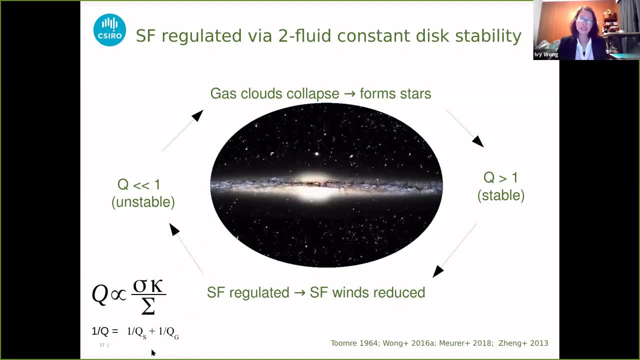 it's sort of the inverse, the sum of your inverse Q stability. So your tumor qu stability is really proportional to your sigma, which is of dispersion, and the epicyclic frequency, which takes into consideration your rotation, and this is balanced off by the surface density or the gravity. so you've got your angular momentum. 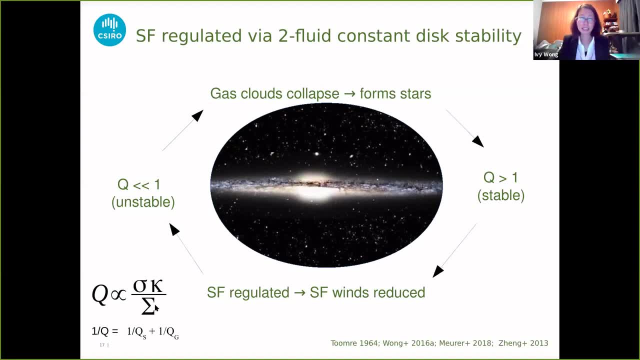 pushing the gas out and gravity bring collapsing the gas together, and so we just keep it simple. we assume this one on q. we assume this q here is a constant of one and a half, and what this means is that as q gets close, close to one, it becomes unstable to star formation. the gas clouds collapse. 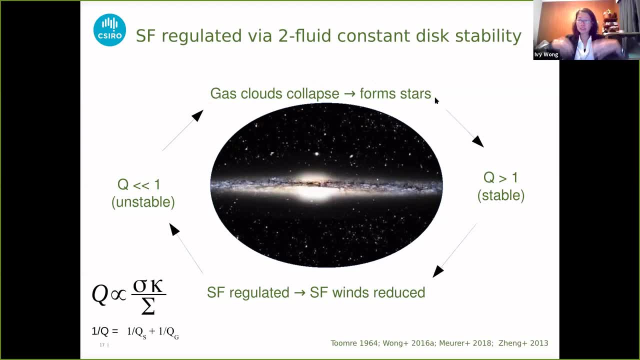 and form stars. and by forming stars the stability goes above one, so it becomes stable against star formation and stops star formation for a little bit, at which point the stuff you know, star formation winds- get reduced and it starts to become unstable against star formation again, and so on and so forth. so this 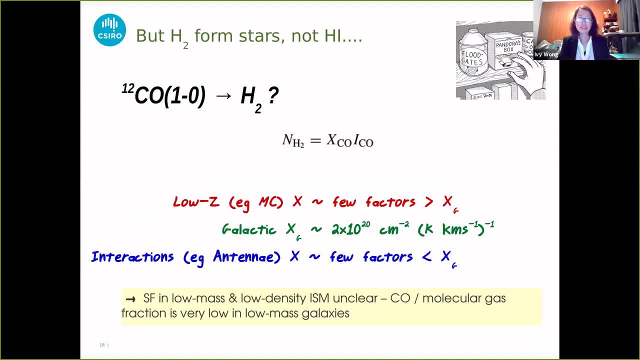 is a simple model that we came up with that sort of works. but what? what i've really not shown you is how that converts to h2, or molecular hydrogen, which is really the fuel of star formation, we think. and this is because h2 is a bit of a pandora's box, as i show you in this cartoon. 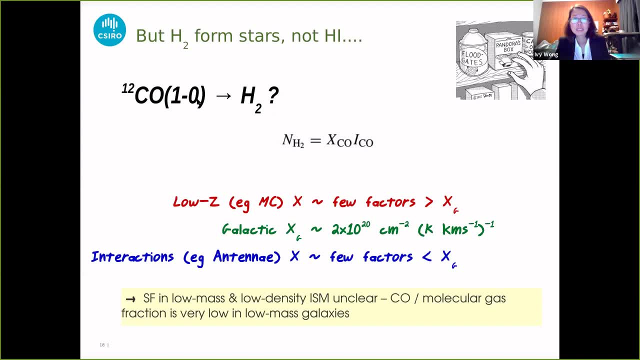 here because we don't observe h2. what we observe is carbon monoxide, and what we do is we then multiply it by the x factor or the, you know the conversion ratio, into to actually infer the h2 column density. we have a nice number that we see here within our 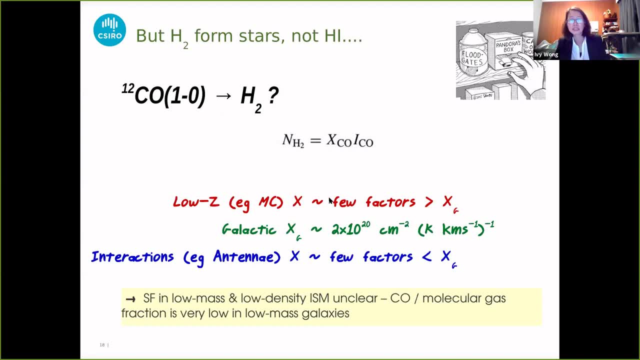 milky way. we know that low metallicity systems like our magellanic clouds are, fact, a couple of factors fewer. so it's you know, it's a much greater x factor and interacting galaxies, or interacting systems, experience an interstellar medium that's, that is experiencing greater pressure, and so 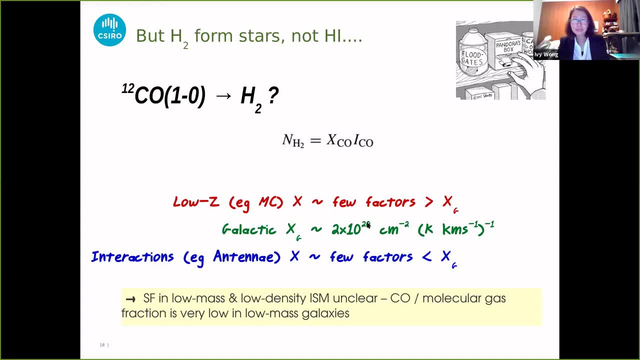 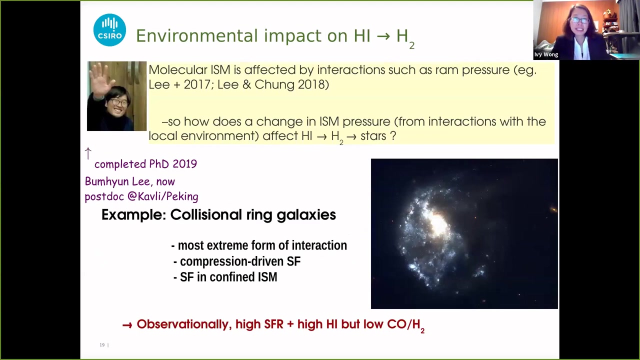 actually this conversion factor goes down again. so it is really quite unclear how accurate or how much we understand of this particular x factor, and this is why star formation is still an area that people work on and there's so many open questions. so how does the environment impact molecular gas? so so far, you've seen the example whereby the 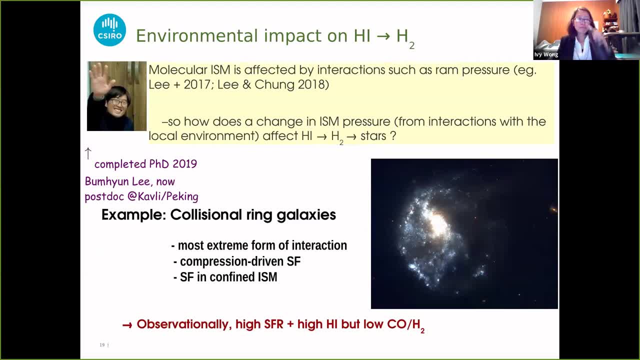 atomic gas gets affected. but here's a picture of um henley, who's now a poster, and he has shown that interactions such as ram pressure can actually sweep out the molecular ism, and so if this is the case, then it means that it has the ability to change the interstellar mediums, pressure and 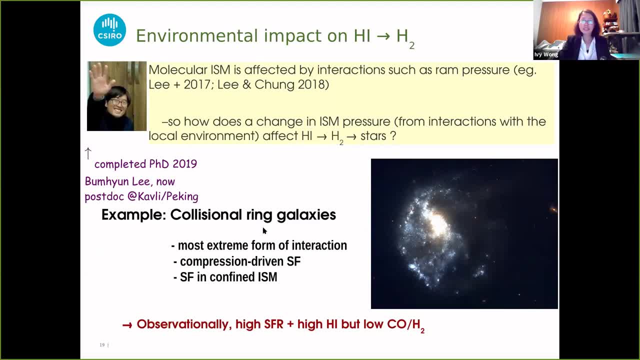 affect how stars are formed. so you can see that this is a very extreme case where the interstellar mediums pressure can actually sweep out the molecular ism and impact how stars are formed. another very extreme case is collisional ring galaxies. it's a very extreme environment whereby a approximately a 10 to 1 merger happens. but 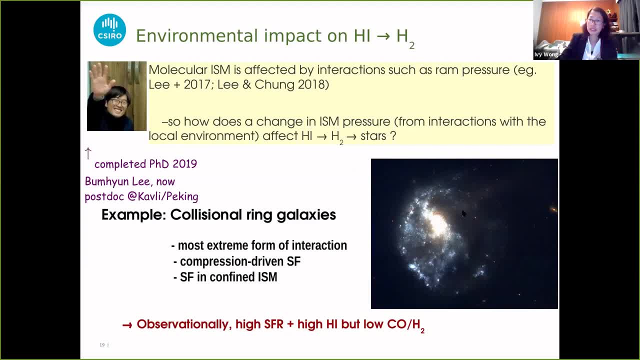 it's not really a merger, it's a drop through collision whereby the, the smaller dwarf interloper, just plunges through the disk of a disk galaxy and that that interaction results in the ism being driven out by the resulting shock wave into this ring light structure and so within this ring light structure. 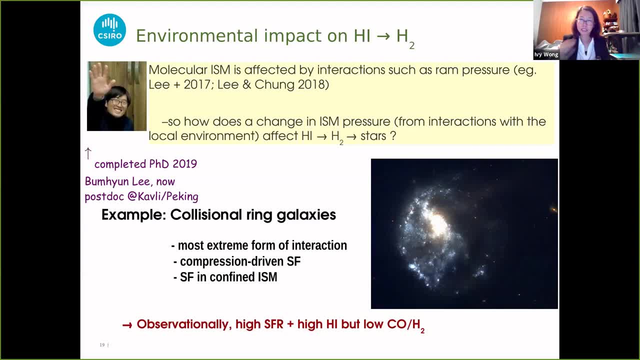 you've got not just regular this star formation process is happening, but rather very much a compression driven star formation in a very confined ism, and so observationally what we see is very high star formation rates located in the ring and high h1, but very, very, very little co or 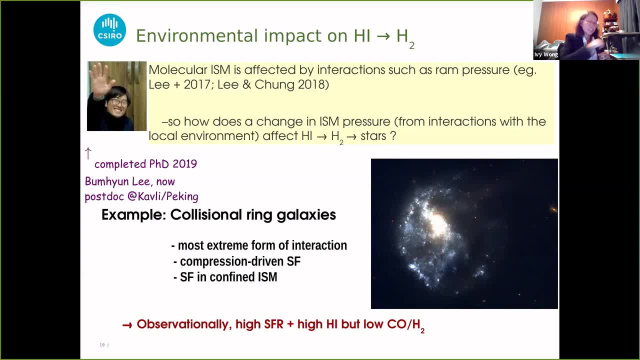 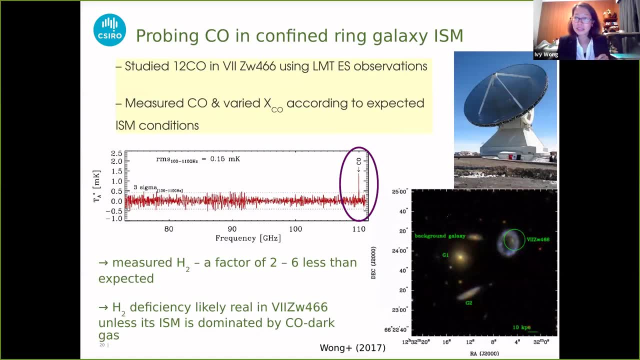 molecular gas. well, this is another one that you see in the ring, when it's significa that a large number of galaxies are replaced with雄 galaxies, and then the second one is the ring galaxies. so what we have here is a single dash millimeter telescope that we can see during its early science. 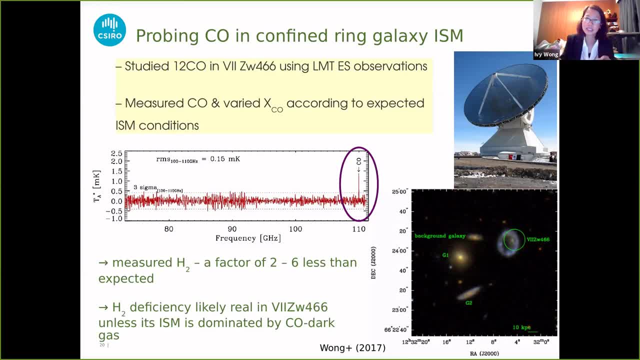 commissioning, and what we find is that, even when we account for the change in exoskeleton, for the change in XCO, we still find a factor of two to six less CO than expected, less molecular gas given its star formation rates, And so the only caveat is that the CO 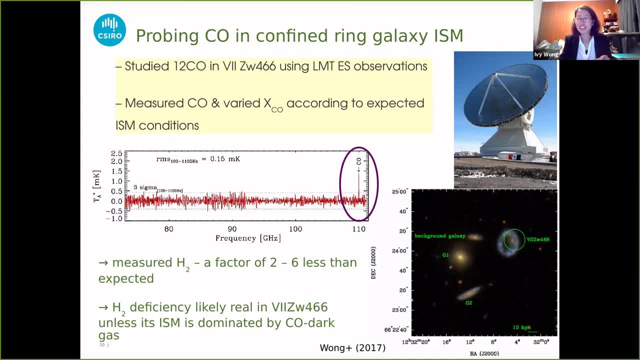 or the molecular gas is hiding in some sort of CO dark gas, and that's actually a fairly unlikely scenario, given the ISM of these galaxies tend to be in very high density regions, because dark gas typically live in inter-arm, very sparse, low density regions. And so what Ring galaxies? 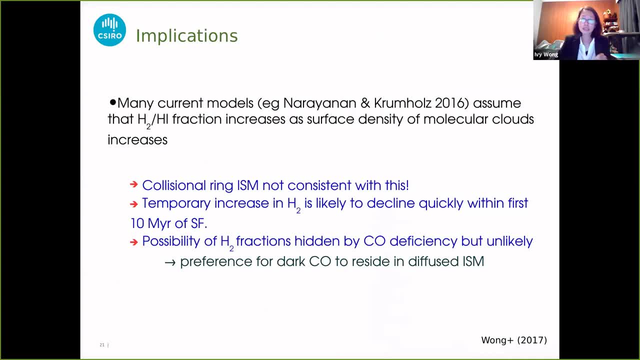 especially collision ring galaxies, are just rare extreme objects. do we really care? Actually, we do care, because most of the current models assume that the molecular to atomic gas fraction increases as surface density of the molecular clouds increases. So this is case in point where 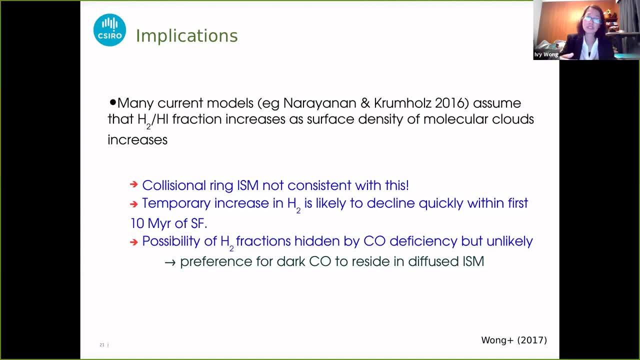 they may be in a very low density region, but they're not in a very sparse low density region. There may be some evolutionary processes where our understanding of the ISM gas fractions- and gas well, the fractions of the gas phases- are not consistent with this And what this means is. 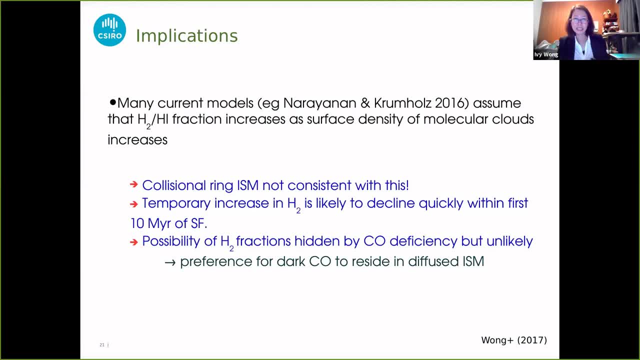 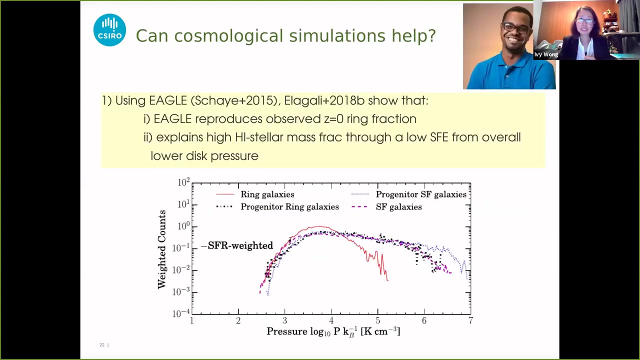 these galaxies may experience a temporary increase in molecular gas and form stars, but then this is quickly declined or destroyed by the proximity of the young massive stars that the actual molecular clouds, And so experience immediate stellar feedback. And so there's one cute little thing, And so here's Ahmed's work. So Ahmed Elagali is a recently completed PhD student. 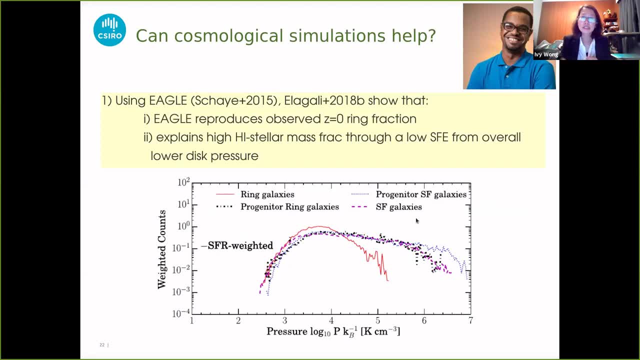 that I co-supervise, And so he's gone into Eagle, one of these cosmological simulations, to see if these simulations could help explain what's happening with these strange galaxies. And what he's found is actually quite nice. He's found that Eagle can reproduce to observe ring galaxy. 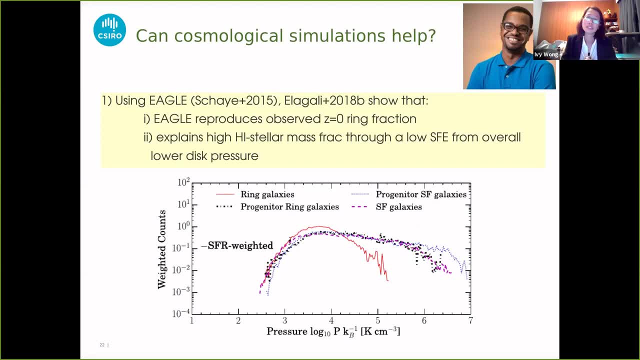 fraction, And so this is significant because this is showing that Eagle is getting the right number of galaxy interactions. And the other nice thing he's shown is that the reason why we observe such high stellar mass- well, high atomic gas to stellar mass fractions. 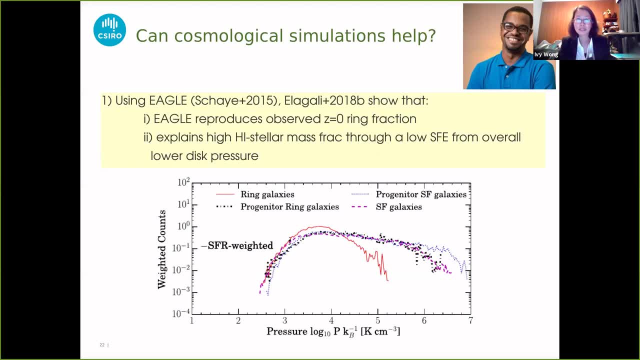 is because these galaxies actually have a very low star formation efficiency, And he's found that the reason they have a low star formation efficiency is because the overall disk pressure is quite low. And so in this plot that you see here you've got regular stuff on galaxies and 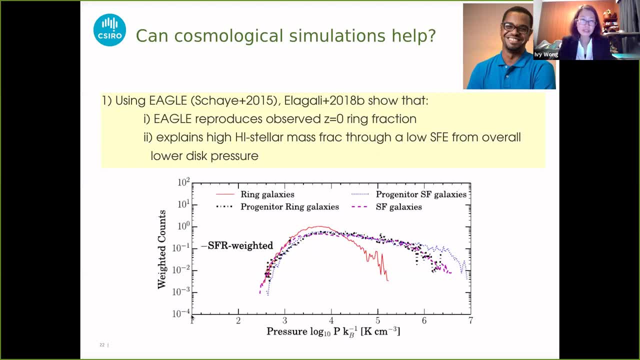 the dotted blue line. So this is pressure versus some. so this is a distribution of pressure of the particles in his simulations. So the dotted blue lines are consistent with the dot dash black progenitor ring galaxies because they are disk galaxies, which is also consistent with regular star forming galaxies. 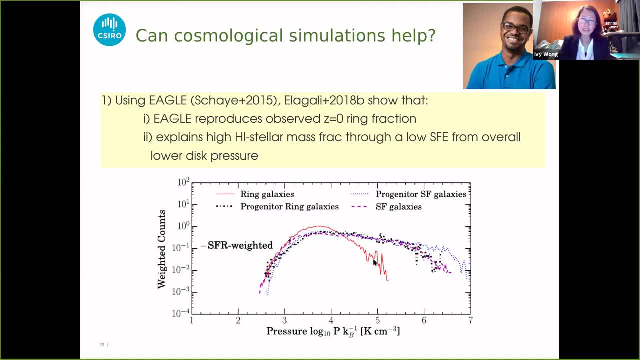 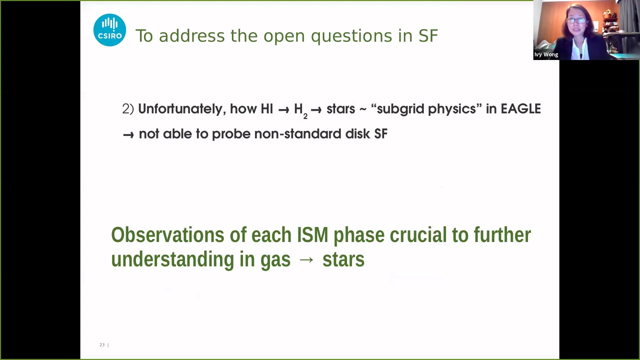 But post interaction, we see the distribution of pressure in these ring galaxies and it's significantly lower than what it was before, thus proving that these galaxies do not have sufficient disk pressure to actually form stars as efficiently as it did before. So this is kind of cute, But unfortunately, because these cosmological simulations 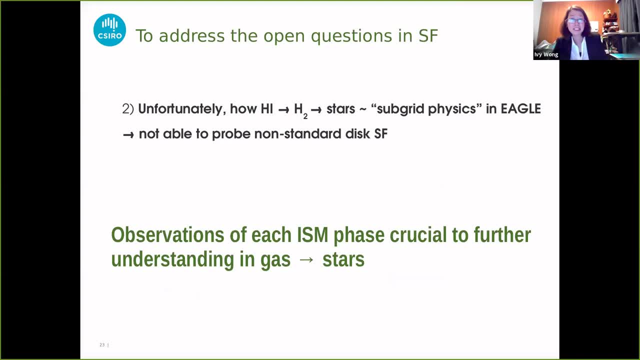 don't have the resolution to actually paint on the astrophysics. it can't tell us how the different phases of gas converts between atomic to molecular and subsequently stars, So we can't actually probe non-standard star formation. And so this is where observations of each ISM phase 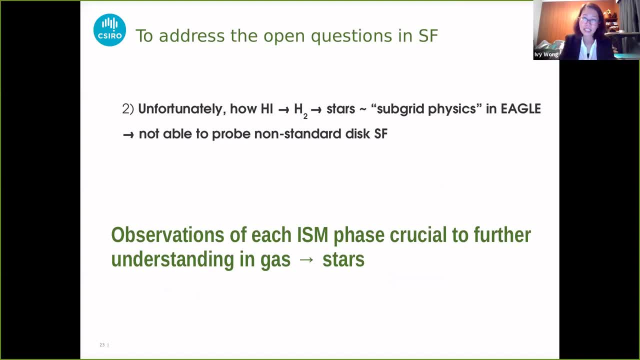 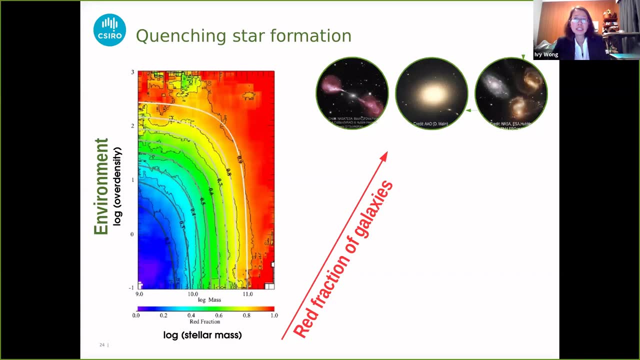 provides important information to our understanding of how galaxies convert gas to stars. So how do galaxies regulate? So this is a very famous illustration by Peng in 2010.. And what we have here is still a mass on the x-axis and a proxy for environment over density on the y-axis, And it's a cute rainbow plot showing. 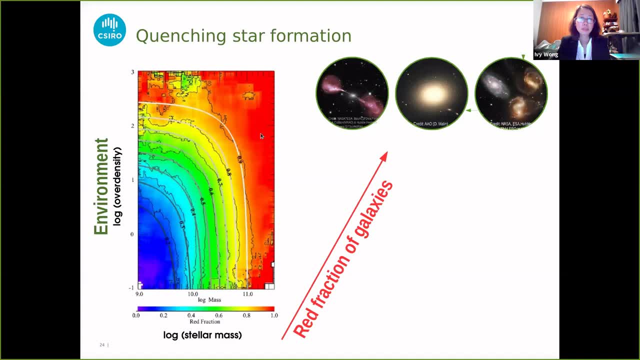 the red fraction of galaxies moving to the top right, And we're down to this. you know the lower three bubbles here, assuming that they're responsible for it. So, first of all, we have a very famous illustration of a galaxy moving to the top right, And we're down to this. you know the lower three bubbles here, assuming that they're responsible for it. So, first of all, we have a very famous illustration of a galaxy moving to the top right And we're down to this. you know the lower three bubbles here, assuming that they're responsible for it. So, first of all, 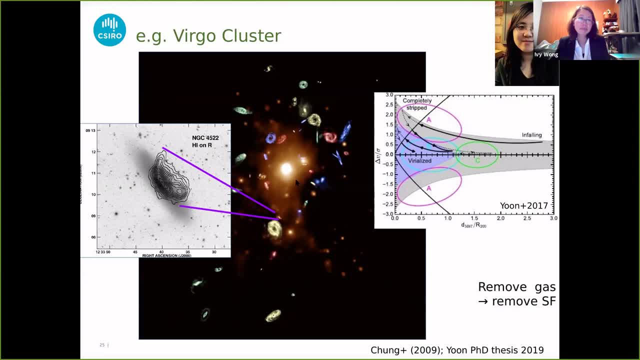 we've got environment. so here's the Virgo cluster and we know that ram pressure pushes out the gas from the galaxy, as you can see from the H1 here of the NGC 4522.. The stellar disk is left completely intact and, you know, nothing appears to be out of the normal But the star forming disk. 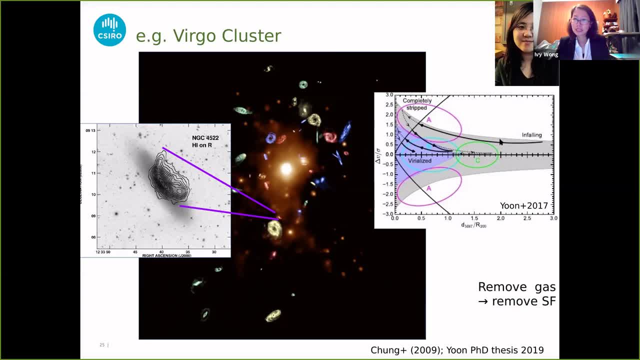 and the gas disk have been truncated. And so here's another piece of work by an ex PhD student, now a postdoc, Hei Nguyen, and he's very familiar with the structure of the galaxy And he's very Hei Nguyen. she mapped the phase space diagram to see what the velocity, the fraction between 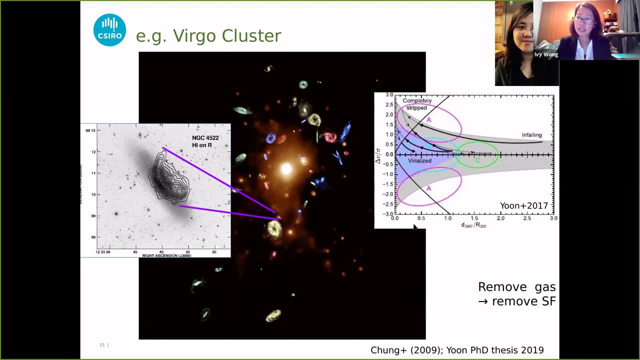 rotation and velocity dispersion is as a function of distance to the core of the cluster. So this is a very- it's a slightly- simplified form of what's happening in the cluster because, as you can see, depending on the location of the galaxy, there are actually two subclusters here that are 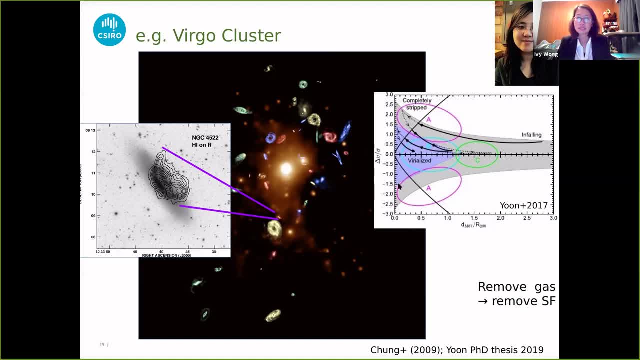 merging into M87. And so this is useful for some of the galaxies that are going around M87, but maybe less useful for some of the galaxies around M49.. But the main message here is that you've got hydrodynamical interactions that can remove your gas and affect your star formation. 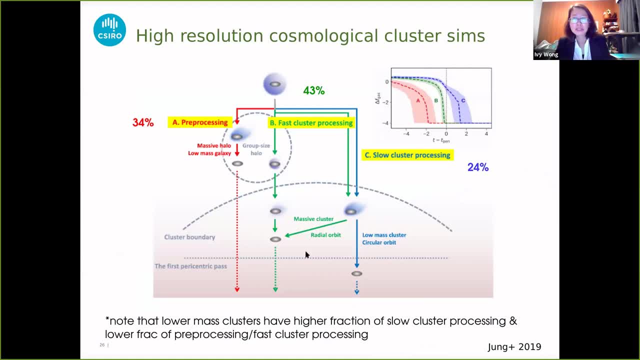 And what do we get from higher resolution cosmological cluster simulations? So this is a set of cluster simulations that have been evolved from the Horizon AGN, but this is a cousin of it that is at much higher resolution. I think they're called the Yonsei high resolution simulations, And what they've found is that 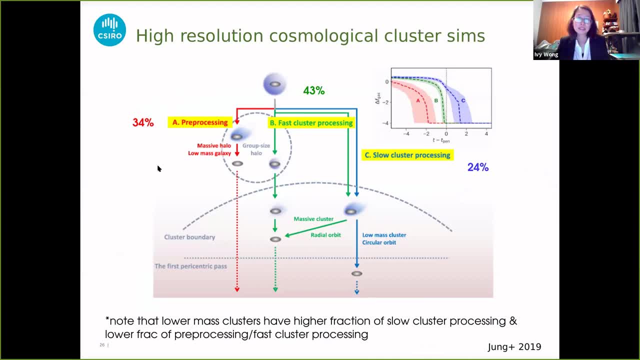 a third of the galaxy is going to cluster experiences pre-processing. So this is environmental interactions that have stopped or slowed down star formation through group interactions, And this is a set of cluster experiences that have been evolved from the Hydrodynamical Interactions. And the remaining galaxies that fall in the cluster can be divided. 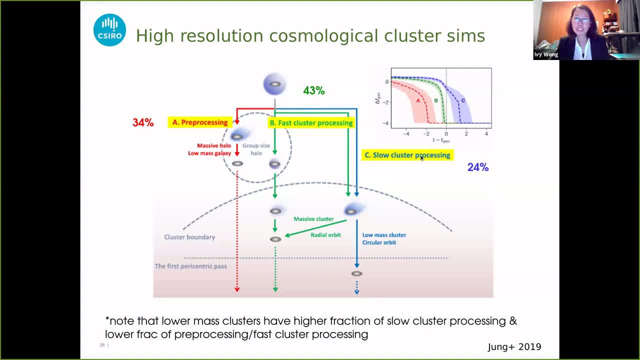 in a sort of one to two ratio between slow cluster processing or fast cluster processing, depending on the trajectory or the orbits these galaxies take before they fall in or the trajectory they take orbiting the cluster. So, as you can imagine, the ones on more tangential 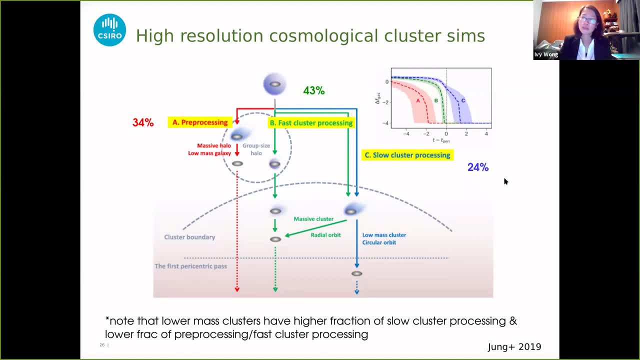 trajectories, experience fast clusters, And so this is a set of cluster experiences that have been evolved from the Hydrodynamical Interactions, And what they've found is that a third of the galaxy is going to cluster experiences- pre-processing or slow cluster processing, while the ones that are more on radio 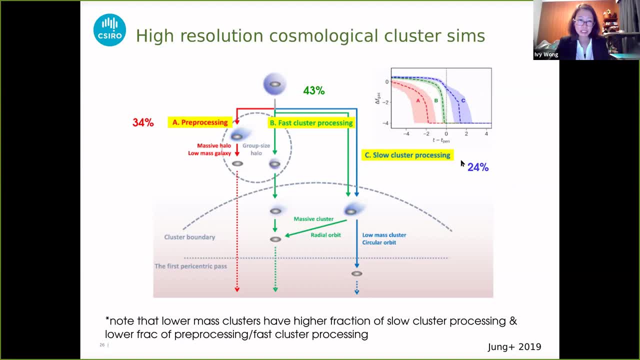 orbits take a longer time before they completely quench. Now I've made a note that lower mass clusters have a higher fraction of slow cluster processing and a lower fraction of pre-processing of faster cluster processing. So a galaxy falling in the cluster may not actually fall into these. 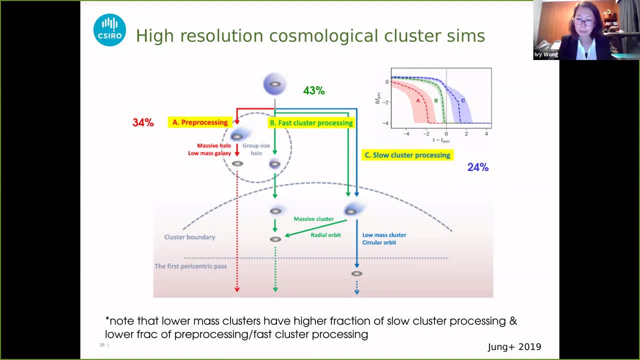 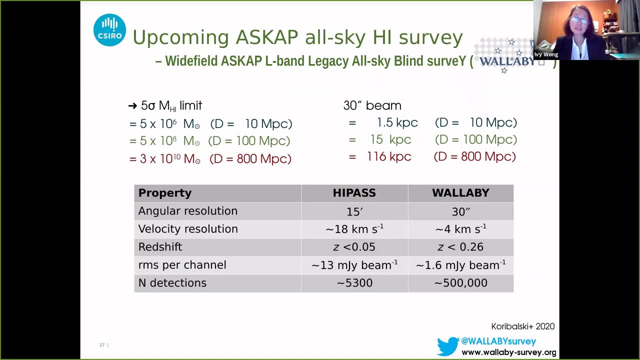 particular demographics, depending on what the mass ratios and orbits are like. So what we'd like to study is to confirm what we find well, not to confirm but to test if our models are accurate by looking at the next generation survey, because High Pass is now about 15 years old. it's high time. 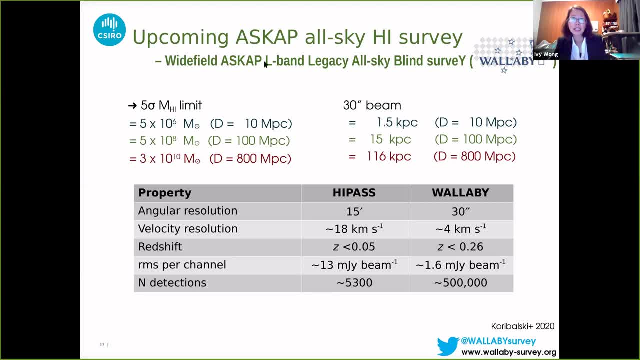 to look at another survey. So with Wallaby, ASCAP is the Australian Square Kilometre Array Pathfinder. we hope to cover our southern half of the sky again, this time at a resolution of 30 arc seconds instead of 15 arc minutes. Have better spectral resolution so that we could actually study. 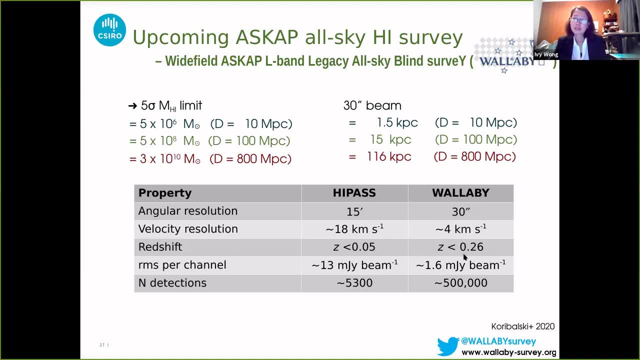 low mass galaxies and dwarf galaxies. We're aiming to hit a ratio of 0.26, but we all know there's some special windows that we can't have thanks to certain RFI bands. so we're hoping to get there, but we'll see what we actually get. So approximately half a million detections in the end. 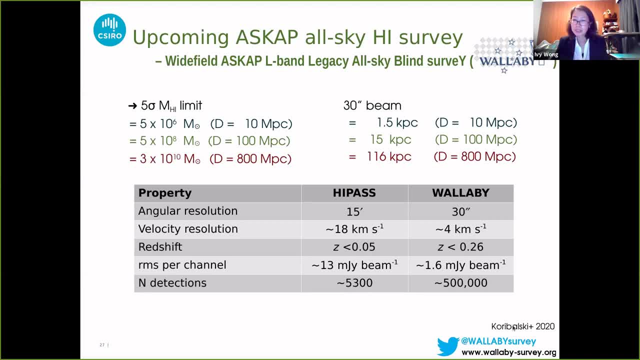 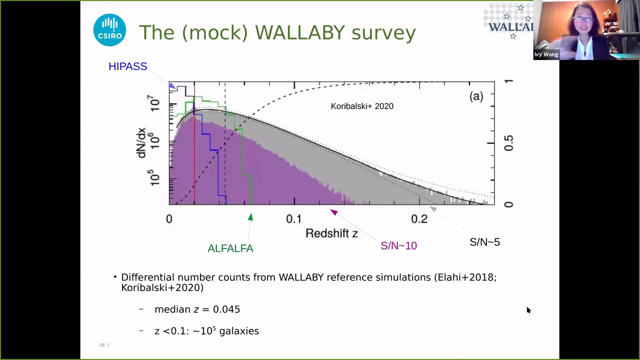 compared to 5000 from High Pass. The paper's out and if you want to join the team, here's the wwwwallaby-surveyorg. It's an open collaboration, so just contact the PI or just submit a. I'd like to join form It's on the webpage. So here's the Wallaby MOX. Once again, the pilot surveys have. 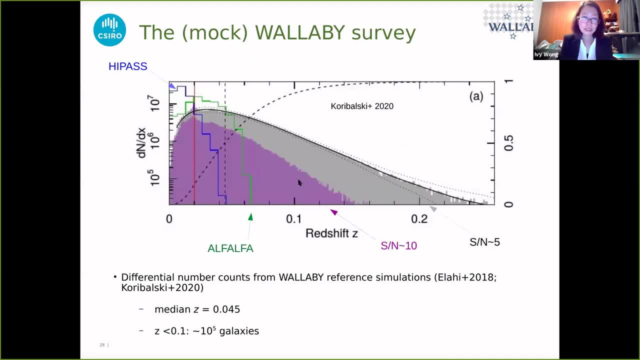 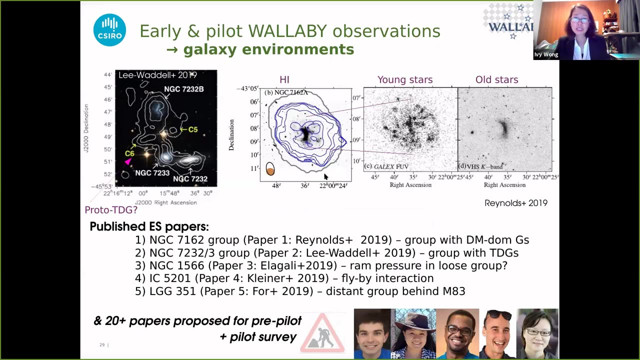 started, so we may actually get more accurate numbers from that, but we are predicting around the half a million mark. So several pilot papers have been looking at processing or evolution of galaxies within galaxy groups, because the majority of galaxies reside in group environments. 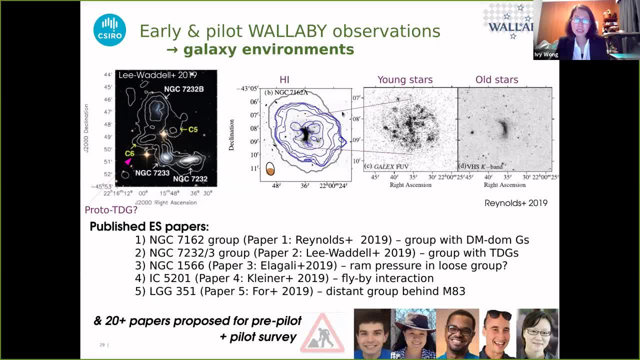 and so we do find very unique systems such as this example that we see here. So on the left, you've got a potential tidal dwarf galaxy. On the right, what we see is a fairly young system whereby the old stellar population and the young stellar population are completely different. 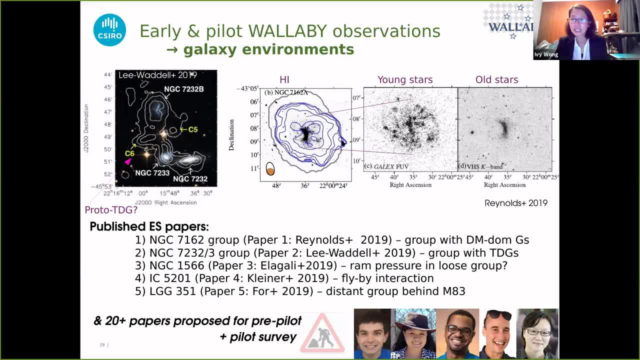 But the H1 provides us with where the gas reservoir is and how much more consistent the young gas is to the gas reservoir. I mean the young stars is to the gas reservoir. So this is kind of cool And the first five papers have been published on the back of our KIND students. 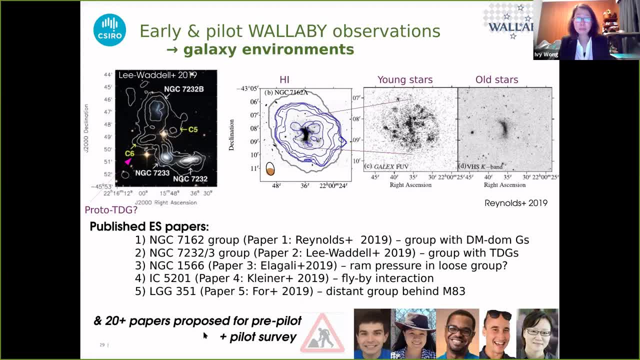 And we've got about 20 plus papers now with the pre-pilot and pilot surveys, And people are hard at work at the latest data sets. But, as you can imagine, the data cubes are now terabyte sizes so they're a little bit more difficult to look at and play with than they used to be. 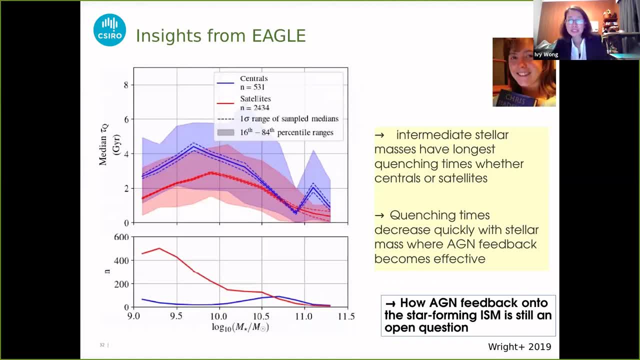 Can we get any insights from Eagle in terms of quenchings by supermassive black holes? So he's a another student, Ruby Wright, And what she finds is that, in terms of quenching of star formations in galaxies, galaxies with intermediate masses have the longest quenching times, regardless of 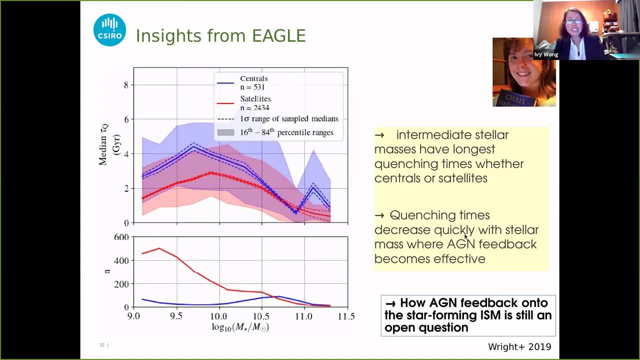 whether they're centrals or satellites, And quenching times decrease quite quickly with stellar mass when AGN feedback becomes effective. So this is all coming from the cosmological simulated models. It is unclear to me at this point if this holds observationally, but we will see, Because 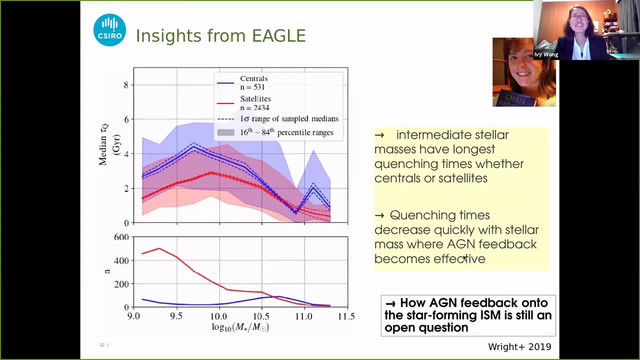 obviously the amount of energy feedback and energy feedback interestingly varies from model to model. So depending on the actual cosmological simulations you use, the amount of energy feedback does vary by a little bit. So that's just me being an observer. So one of the interesting questions, for observers at least, is how does AGN actually feedback? 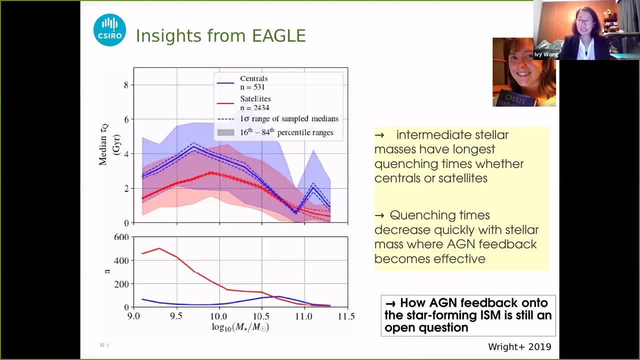 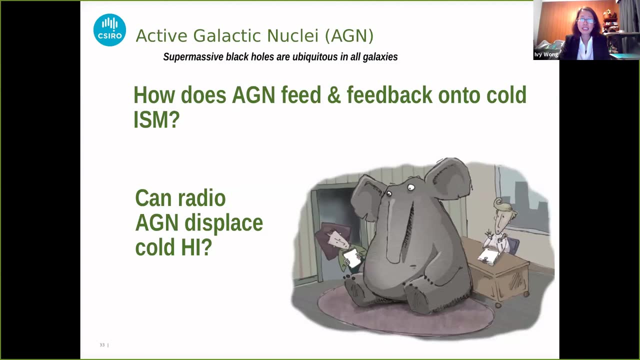 Do we have direct evidence for this feedback, especially the mechanical energy feedback that is imparted onto the interstellar medium. And so the big elephant in the room is: how does AGN feedback feedback onto the cold ISM? Does it even displace the gas? So we've seen some 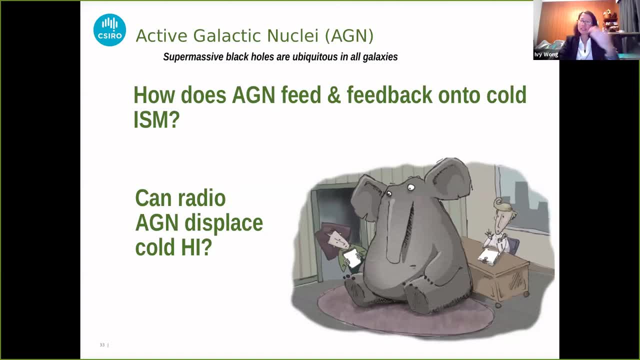 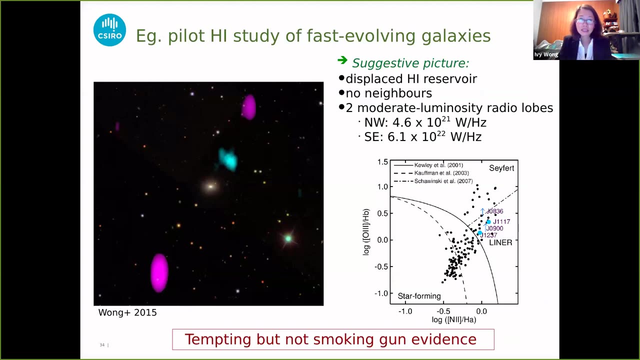 tentative evidence for CO gas now in a handful of galaxies being displayed near the core of the AGN, or at least in the line of sight of the AGN, because it's an absorption system. But can it actually affect the atomic gas? So here's a quick, bizarre galaxy that I reported on. 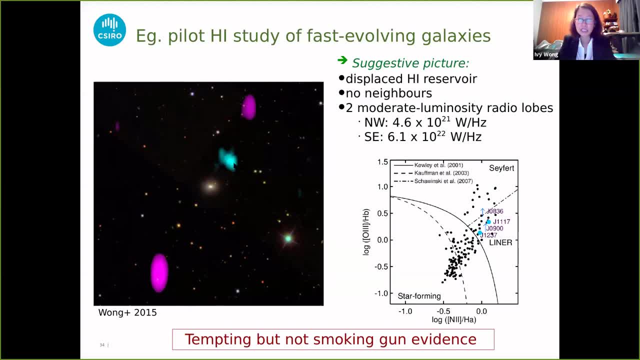 So this is not me suggesting that this little blob of H1 gas has been blown out by AGN activity. It's just a tantalizing picture that we see here of a spheroidal whose H1 is out here sandwiched by its two, by its two radio lobes. This is really what we see. We don't know how it. 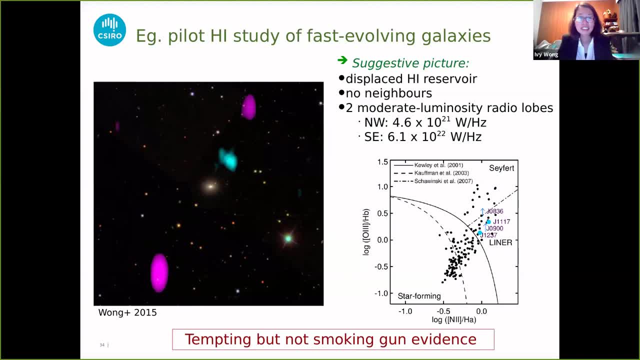 got there or if it had anything to do with the radio lobes. but so far we haven't found a companion galaxy to this particular case. So we're still looking into what's happening to this particular galaxy. And what's interesting is that if we were to study a stellar population, 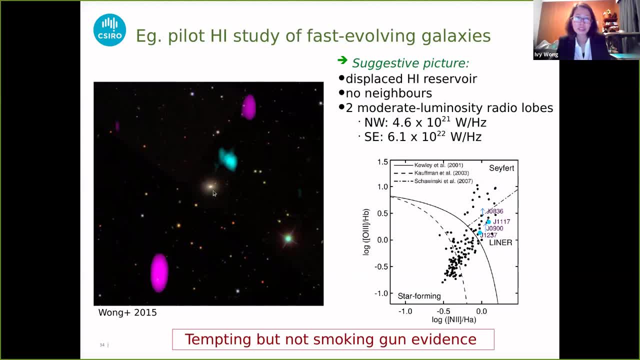 the quenching time was about a giga year or so, So it experienced a very fast star formation shutoff. So I really don't know how representative such a bizarre case is. I'm just showing this is what an observer can see. So what's nice is that with the current BASS, 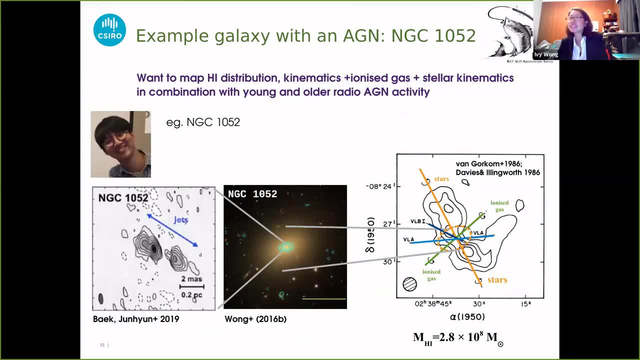 survey that we're doing. so this is the SwiftBAT AGN spectroscopic survey. So SwiftBAT is a space probe in hard X-rays, and so you're wondering: okay, you've just jumped to hard X-rays. Hard X-rays is really cool because this is the mission that comes right down from the AGN. 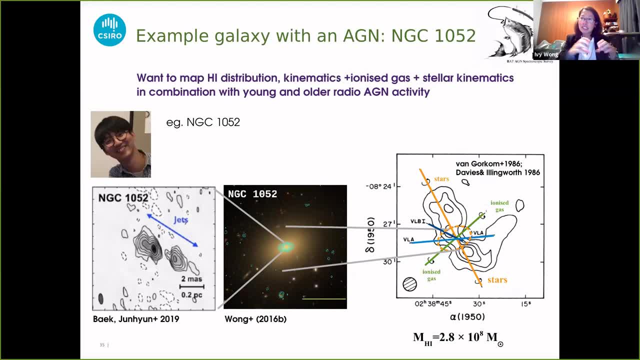 much closer to the black hole than the soft X-rays. So the soft X-rays come from the crescendo. This is what we think it comes from, and so what these nearby galaxies are doing are that there's some restarted AGN mission, I mean Allegian activity, as in the 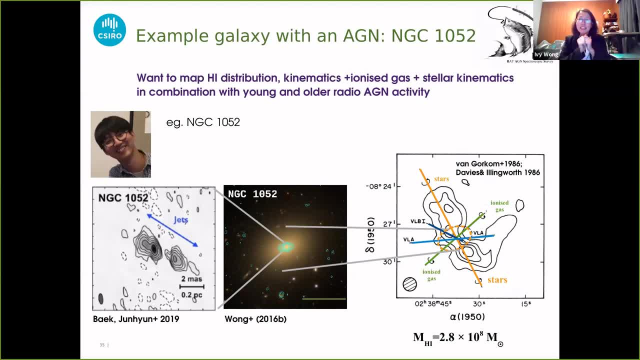 activity as inferred by the presence of the hard x-ray. So what's happening to these galaxies right now? So what my mission, or what I like to do, is to map the gas distribution, And so in a few cases, people have done this, for example, NGC 1052.. So this is Chunhyun Becks. 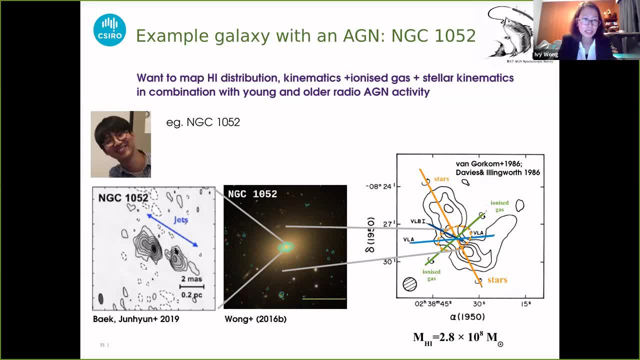 one of my other co-supervised students. He's now a postdoc at CASI, So he's used the Korean VLBI network to look at the- yeah, the milli-arc second scales of the radio jets within this particular spheroidal galaxy. So the first emission, so this is 1.4 gigahertz emission. 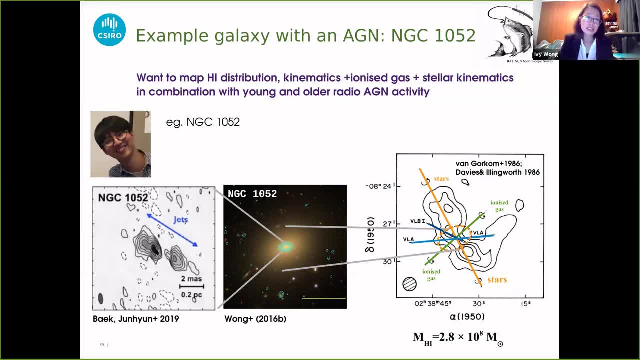 shown by the cyan. If we could do VLBI on this, we could see down to the Parsec scale or sub-Parsec scale jet for what's happening to this galaxy. But what's really cool is that in the 80s, 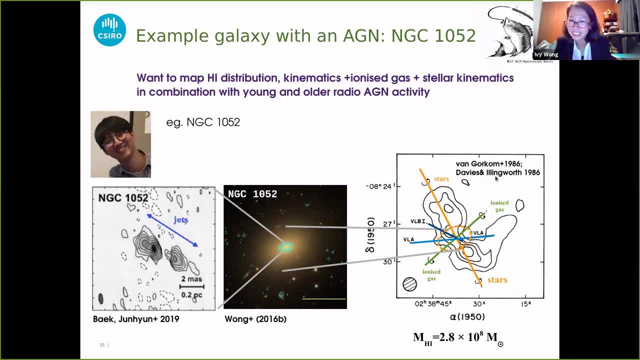 this is the first emission that we could see. So what's happening to this galaxy? So this was a map by Jacqueline Van Gogh and Davis and Illingsworth, And you've got a complete orientation shift between the VLBI jet, which is this dark blue line, to what we see in the VLA. 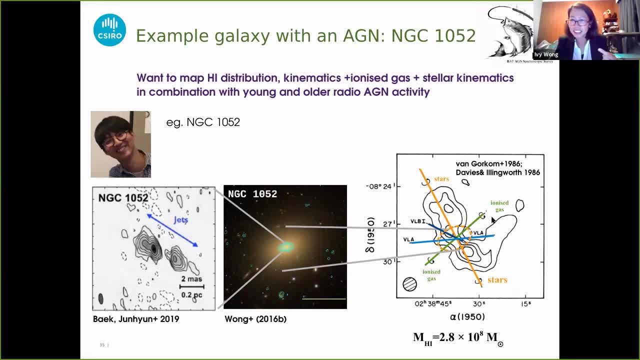 And the ionized gas is actually rotating in a different direction to what the H1 and the stellar body appears to be. So this is one of the other bizarre cases, And so the idea is if, given the number of galaxies we now have with BASS, how common are? 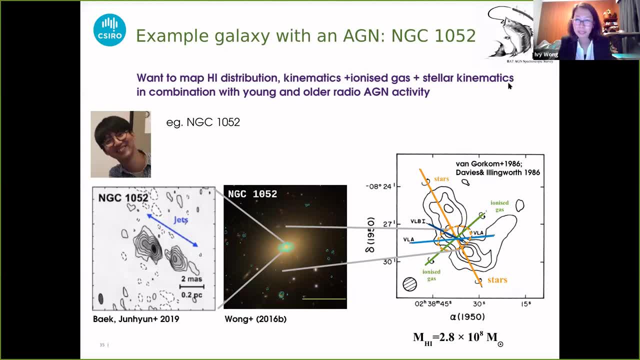 these. So we have a pilot survey with the Compact Array now, but a bigger program with the VLA, And so fingers crossed that we can get down to what's actually happening to these particular galaxies, Because we're at a stage whereby we realize that we're no longer talking about. 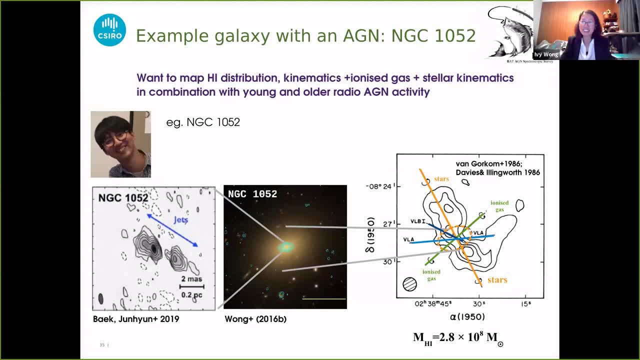 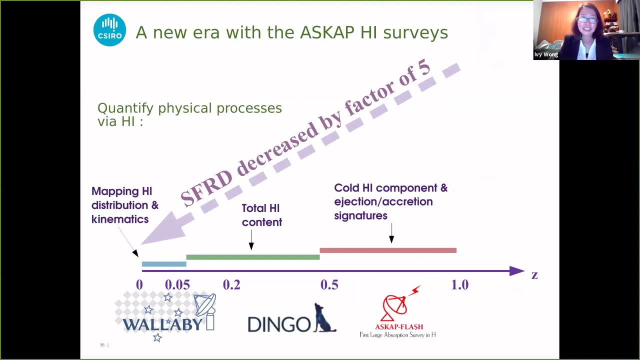 whether galaxies are AGNs or star forming, We now understand that everything's co-evolving, And so it would be good to piece together the details of this particular puzzle, And so I've shown you a lot of bits and pieces in star formation and galaxy evolution And what's. 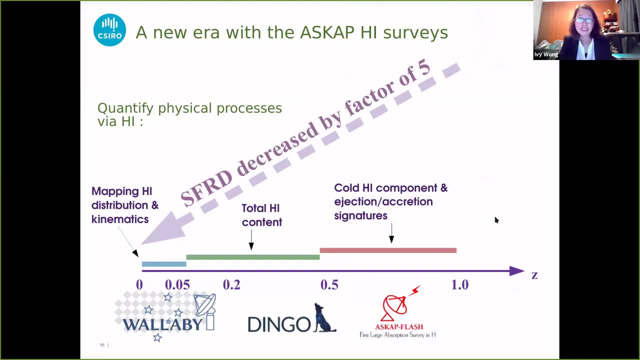 really nice is that the next generation ASCAP surveys will help us further our understanding on quite a lot of these different science cases, And so VLBI will give us once again the low redshift mapping of H1 distribution kinematics. And then we go up to Dingo. So, oops, clicked again. 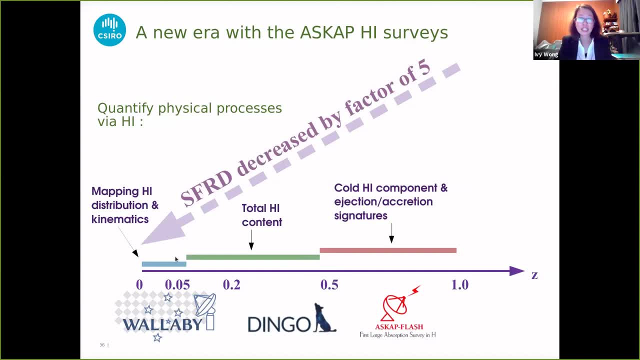 So Dingo is more of a pointed survey where they aim to go up to a ratio of 0.5. So there's similar ish to mighty H1. And then at Meerkat, Ludumo would have direct mapping on the very small. 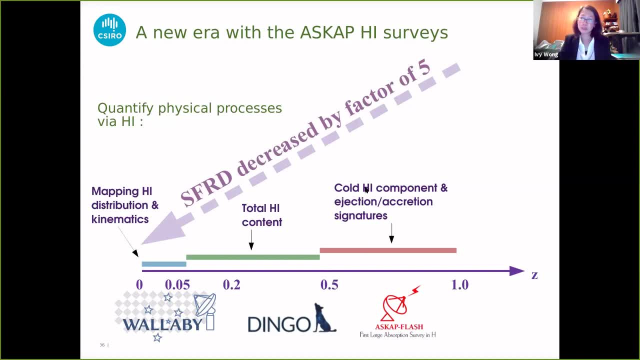 pencil beam, But we also have ASCAP flash, which is an absorption line survey with ASCAP, which will go out to about redshift of 1.. And so, at this point in time, this cosmic star formation rate density have decreased by a factor of 5.. It'll be interesting to know what happened to the gas. 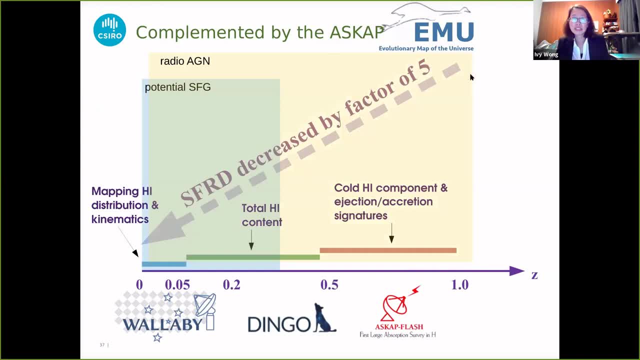 And what this is complemented by is the All Sky EMU survey and radio continuum, And it provides us with the potential to measure star forming galaxies up to a redshift of about 0.3 or so and radio AGN out to redshifts of 4 or 5.. 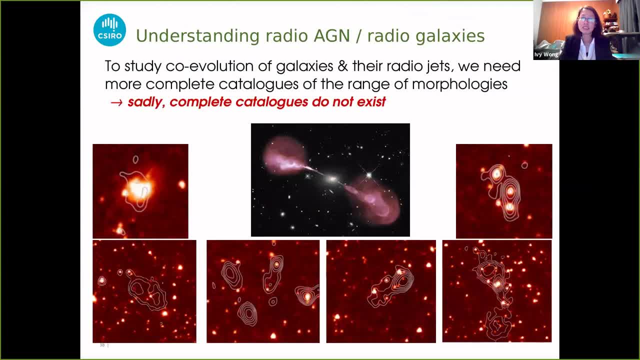 But unfortunately we really don't understand radio AGN very much at all, because it seems to work on slightly different timescales to the optical quasar mode of AGN or the radio mode of AGN. And what's worse is that even though in our ideal dreams we would have a nice beautiful VLA set of radio jets Overlayed on HST imaging- 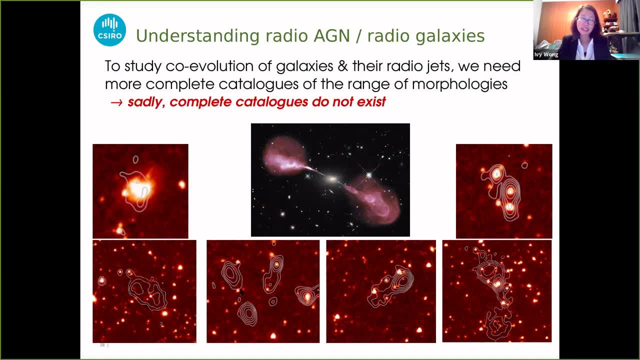 the reality are blobs and blobs, and it is difficult to understand the evolution of these blobs if one is not able to even disentangle where these blobs come from. and so what I mean is that if you, if one were to see this particular hourglass structure, where is its host galaxy, or which host galaxy is it coming from, or is it a? 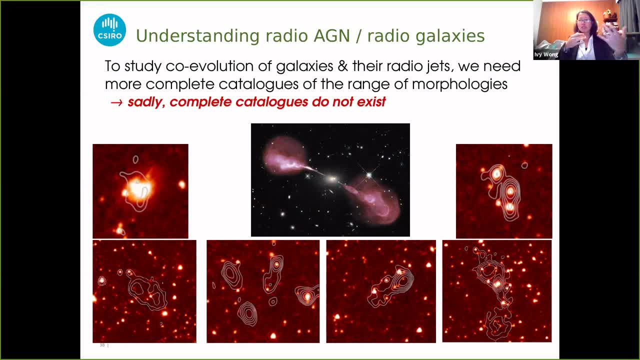 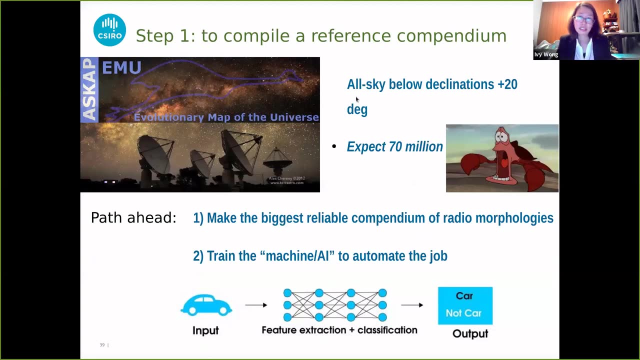 multitude of host galaxies. so, unlike H1, we do not have the extra third dimension or radial velocity, and everything's just projected on the sky, which is slightly, slightly frustrating. and so when one were to want to cover the entire southern sky, we would expect 70 million sources, and it's estimated 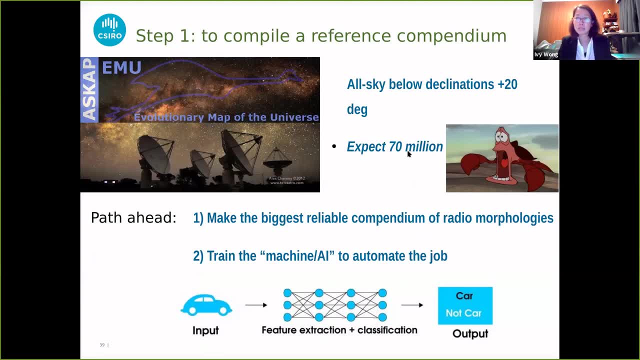 that 10 of these will not be easy compact point sources for cross-correlation, and so what we really need is to create a big, reliable compendium of radiomorphologies and hopefully train some of these machine learning tools to help automate the job, so that at least if we could reduce that 10 percent of. 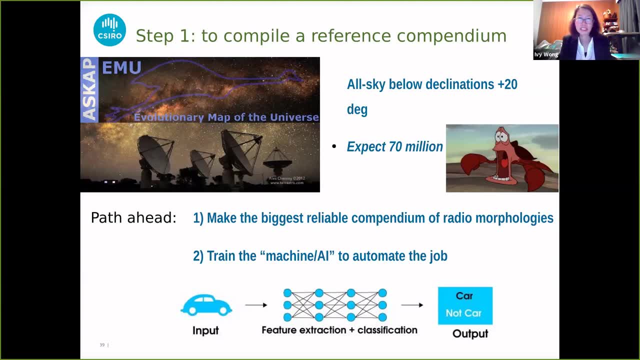 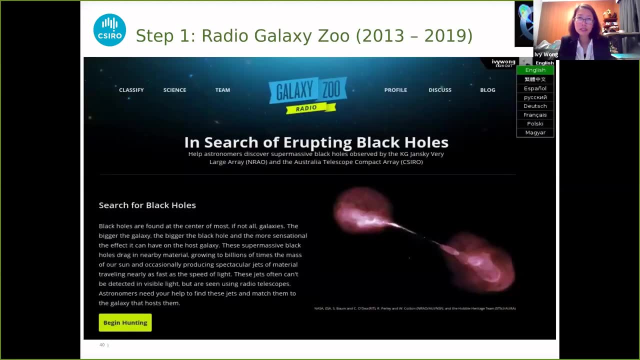 sort sample that require eyeballing or human intervention, down to about a sub one percent, this becomes doable. so we ran radio galaxy zoo, which is a citizen science project run online internationally to look at the first and atlas sample of extended radio sources. it's available, it was available and it's available on the internet. and it's available on the internet and. 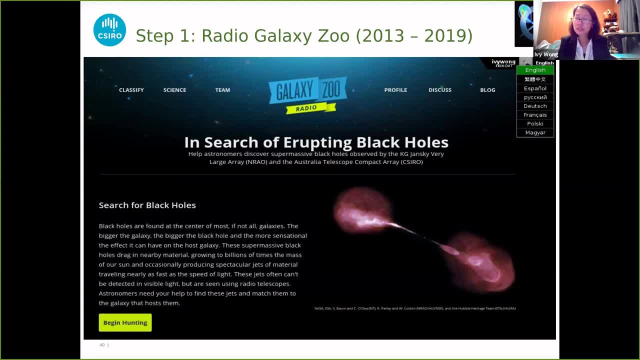 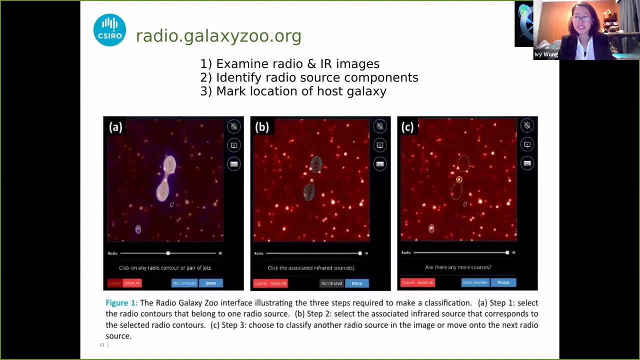 available in eight languages. currently it's in phase two, so the radio galaxy zoo project is now focusing on lofa. if you're interested in participating, you can google for lofa zoo. it's called lofa zoo and the idea really is to identify associated separated components with 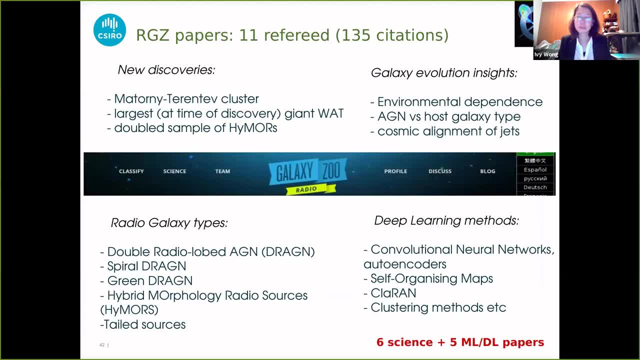 the host galaxy. it's very, very simple. the majority of this is based on the first survey, and it's quite actually heartening and surprising that we could have enough discoveries to publish several papers. so that's fun. what's really fun was we could then test our pipeline, which wasn't perfect, but we could. 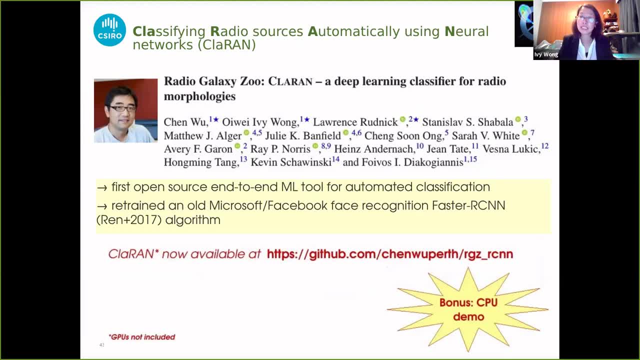 create a little prototype to try to automate the process of classifying radio galaxies, and so this is the github link. if one or you can also google claren again. it's quite easy, and the nice thing is, we now no longer need radio galaxies layers, and we just need them to take a master in the data system. 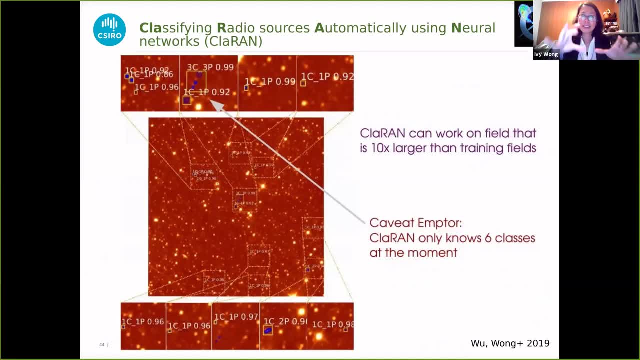 for us to be able to pick up the data and then make some designer calculations and then have them longer need to create tiny cutouts in specific regions. We could just feed in an image to the to the piece of software and it would identify where the sources are, regardless of how many. 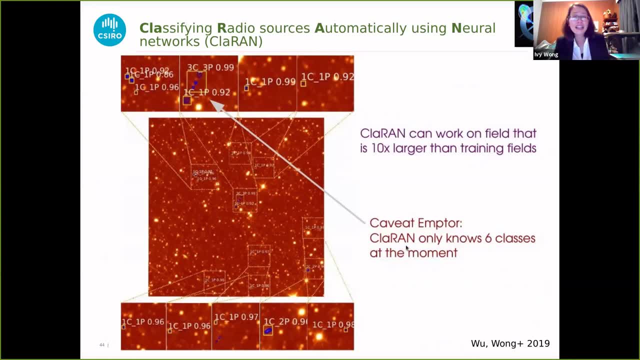 sources you have in there. So the only caveat is our prototype only recognizes six classes, and so we very honestly show you the the wrong answers we get, such as this particular case where we know there should be four components to this radio galaxy, but CLARIN hadn't really gotten up. 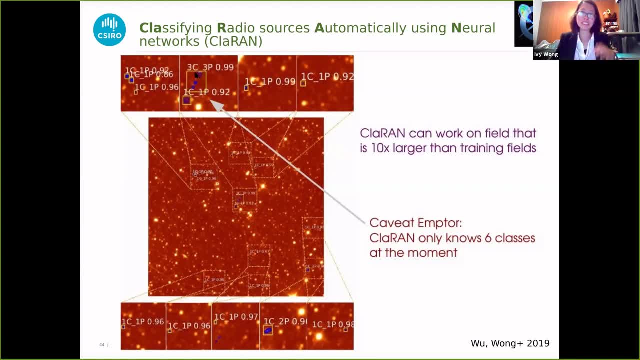 to that level yet. so it thinks it's a one component and a three component source next to each other. So what you put in is what you get out. we continue to work on this, but it's out there, the code's out there, so if anyone's interested in forking it and training it, feel free. it's completely open. 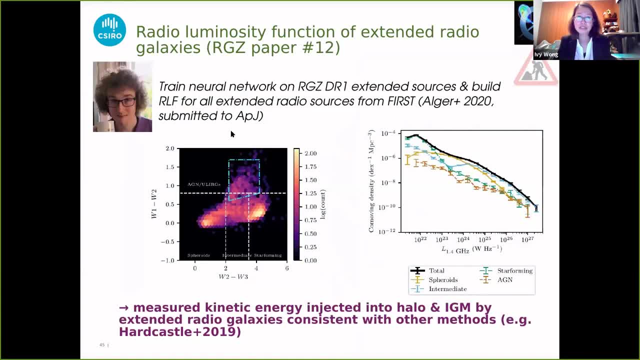 What's fun was my other PhD student, Matthew, was able to then train it on radio galaxy morphologies and then unleash it across the entire first sample of extended sources to create fractional luminosity functions from different populations as suggested by their mid-infrared colors. so that's a bit of fun because he showed that by and large- okay, the very high. 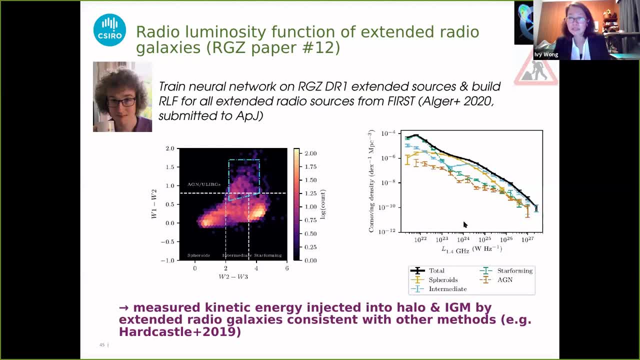 luminosity sources would be dominated by what you'd expect, which are mainly the spheroids. but then what you'd one doesn't expect is this double bump from what we term as intermediates. so this is the intermediate region. so we know that ellipticals and spheroids live on this left corner. 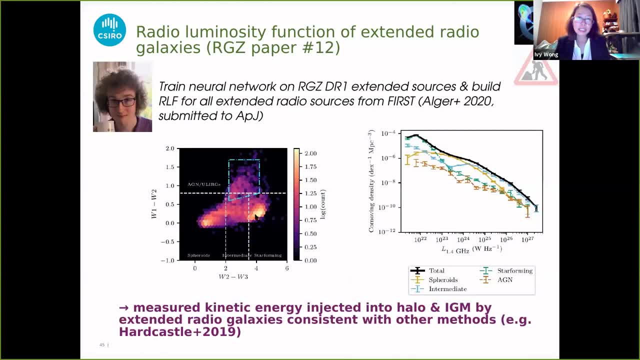 star forming the start. oops, oh yeah sorry. starburst galaxies live in this other corner and eulergs and quasars live up here in this blue box And in this intermediate region. we see a nice mix. that's highlighted by the sign and what I'm trying. 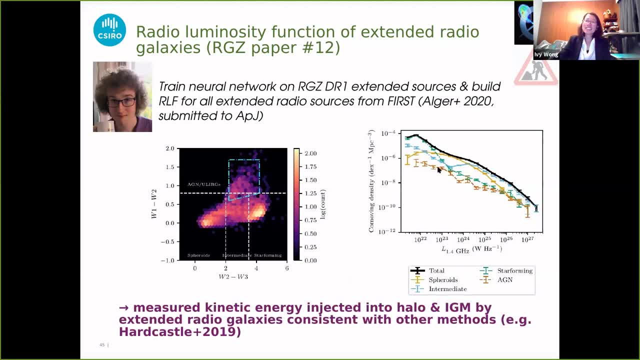 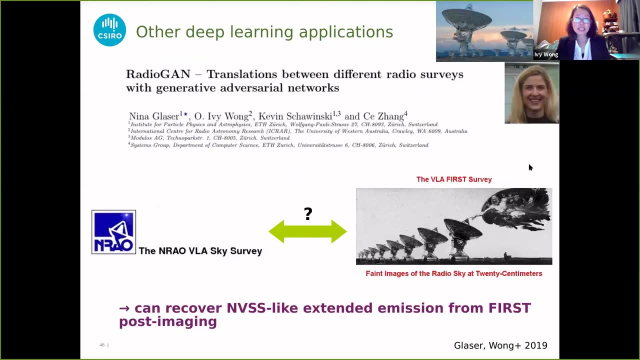 to highlight with my mouse now, and so this is suggesting that there is there. there is a very, very large population of galaxies, for which star formation and hgm is equally important, and so this is nice and consistent with current studies. another cool deep learning application is the translation. 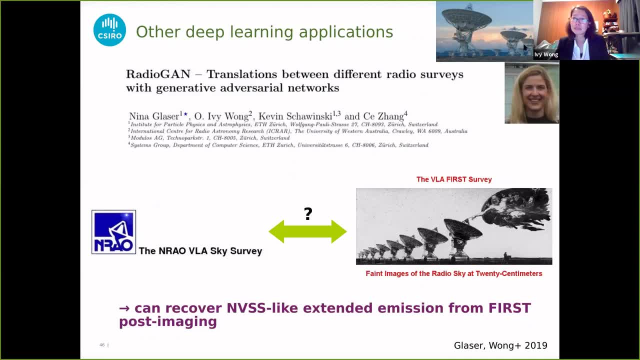 between different galaxies. So in this case we have two different radio surveys. as I was mentioning before, depending on your array configuration and distribution of baselines, you could have better resolution or better sensitivity. but what this means is that if you provide sufficient information to your little, 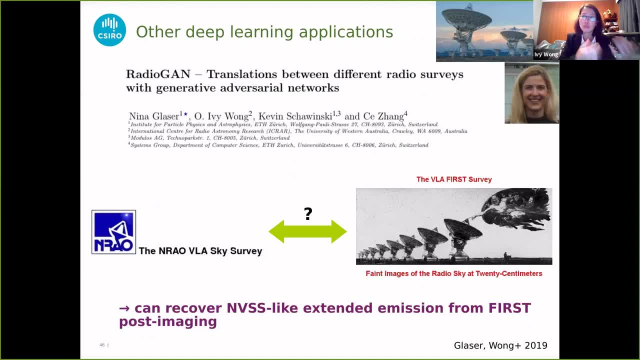 machine. it would learn the characteristics of your noise from one array configuration to the other. so in this particular case we confirmed that we are able to recover some of the diffuser emissions, say from first, that have been resolved out by the first survey, compared to the nvss survey. so this 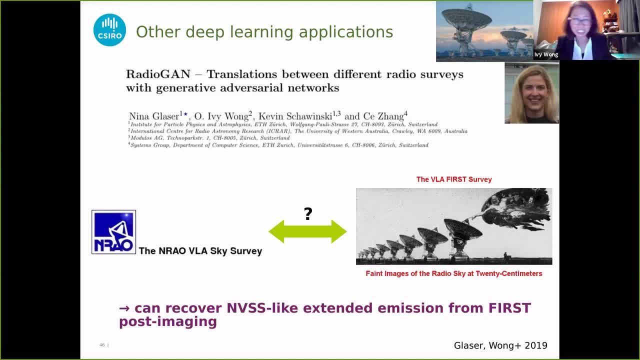 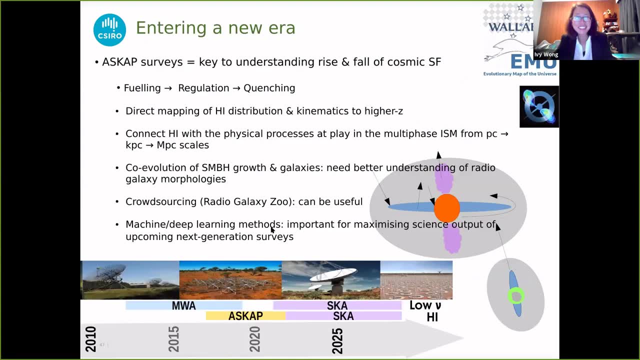 is kind of cool and, as you know, I come from an h1 background, so recovering extended emission is one of the goals that I hope to do so, and with that we are truly entering a new era- well, worldwide really. but in this particular talk I'm focusing mostly on ASCAP, because the 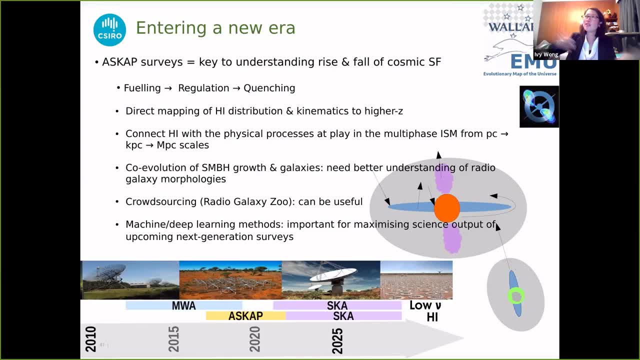 phone is important to us because this is the telescope that's within the state whose borders well it's. I don't have to cross borders to get to this particular instrument. let's just put it that way. and even on this one instrument alone, I think we're going to gain a lot in terms of 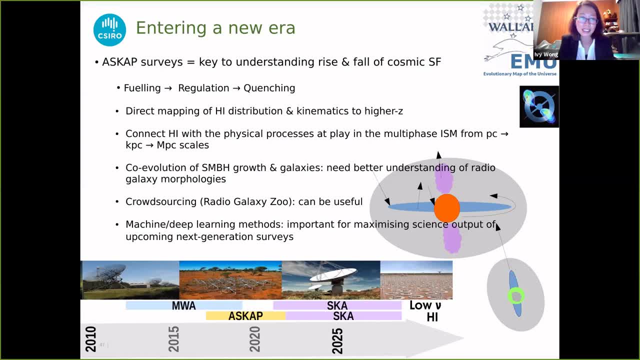 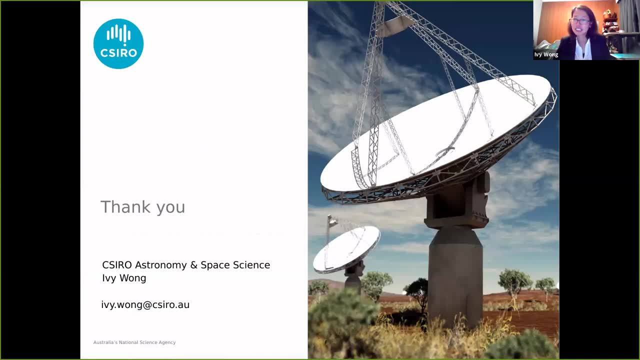 understanding how the gas maps to the stars and how subsequent galaxies evolve. So thank you very much for your patience and time and any questions. thank you, Ivy, we'll take some questions. so if firstly, students, if you have any questions, please either unmute yourself or raise your hand. yes, in here we'll. 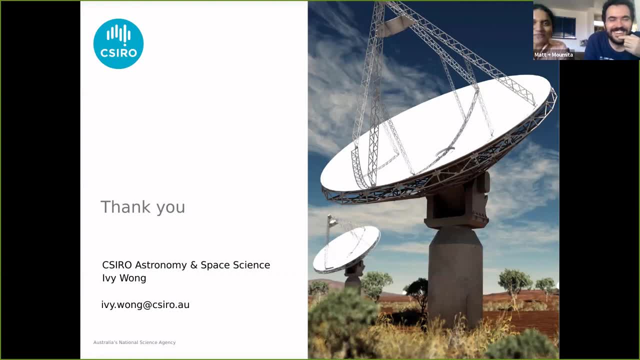 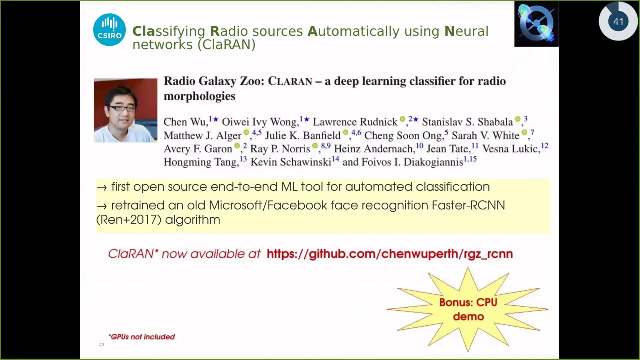 come to you just giving the chance to other students, if you okay. um, I don't see anything. so, okay, Inje, you can go ahead. so I mean, my question is: can, like one of you, give some kinematic information of the galaxies, like their spin, such rotation and such? yes, for the nearby. in which way? how can I, if I'm 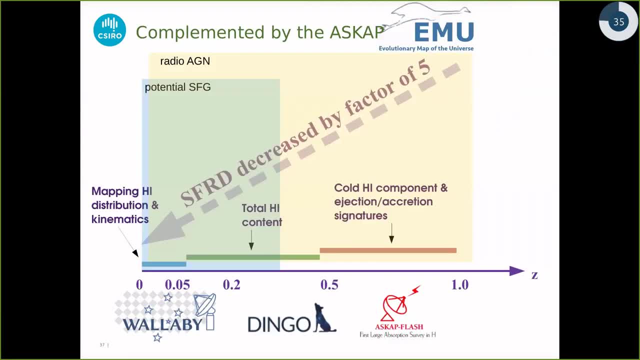 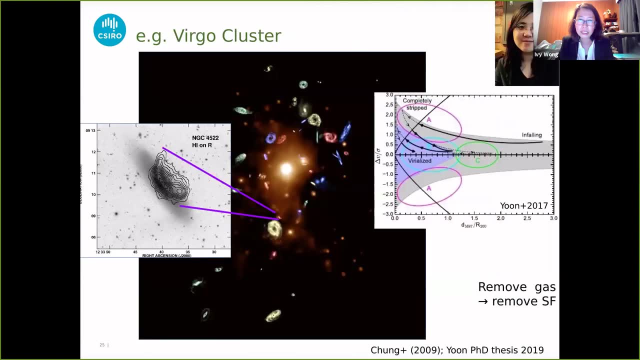 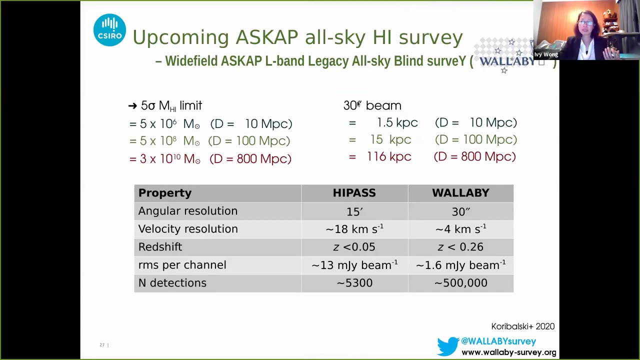 interested in like a galaxy spin and their axis and so on. how can I get it? so you let's go back to h1 galaxies. so if you're interested in the spin, what you need is a resolution of a couple of beams. so this is the synthesized beam. 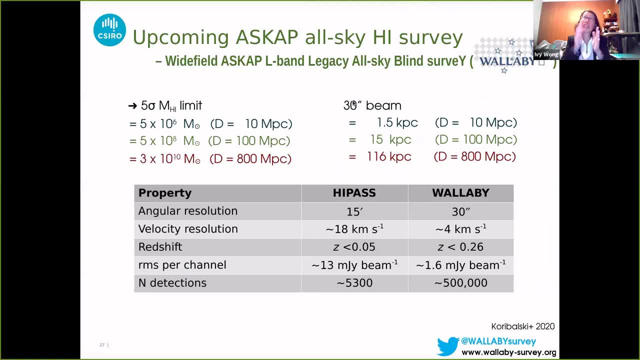 size over 30 arc seconds. if you have a minimum of three to four beams you can. you can model it with a rotating disk, so there'll be a lot of degeneracy. so ideally you want about eight beams across for a properly resolved kinematic disk modeling, but you can get away with four beams. so the data that 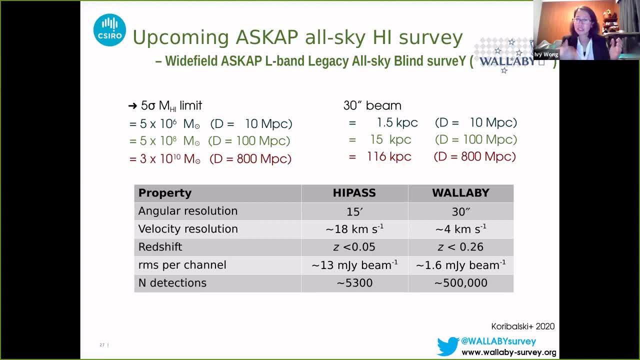 comes through through is a 3d data cube with velocity on one side. so if you know the inclination and position angle of your stellar component, that could help you constrain which what the the true position angle of your kinematics is. but if you work on diabolical galaxies like the ones that I work on, they may not be. 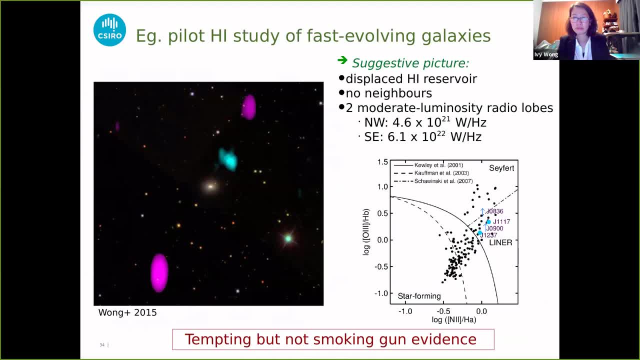 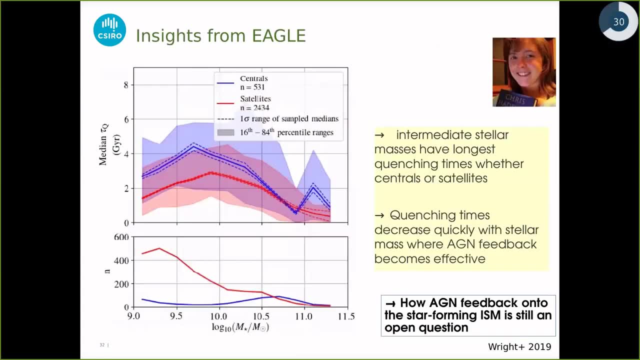 aligned with your stella disk and so it depends. okay, I see, thank you, yeah, if that makes sense. yes, yeah, cool, any other questions? oh, sorry, okay, Rose and Shilpa, I'm sure poto may be. Rose, go ahead. hi, I got maybe one・ wrong, is it? May I say? 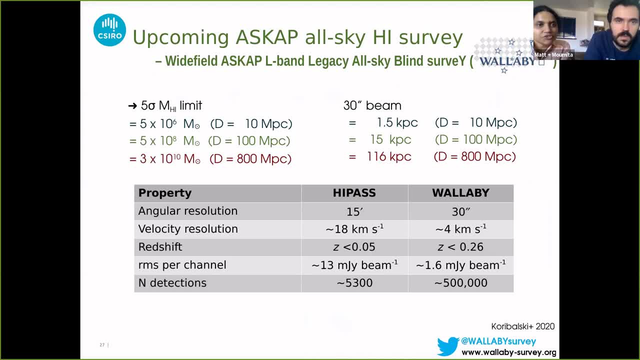 something right. so if you were to all of us, like I know in, like a typical, I was wondering that strange galaxy or situation. you actually just had it up on the slides again where the H1 is completely offset. Do you have redshift measurements? 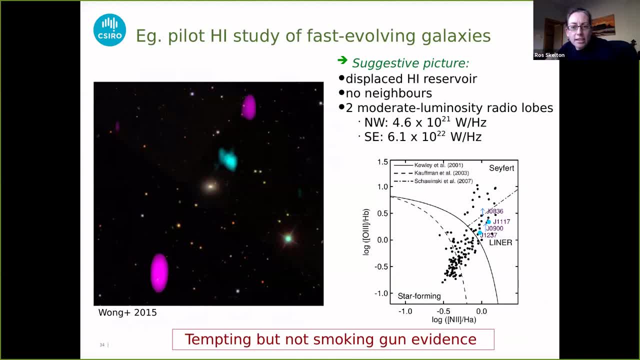 You know, is the gas definitely at the same redshift as that galaxy nearby, Sadly, yes. So we have SDSS spectroscopy on this particular, on the stellar component of the galaxy, And because these are pointed observations, we're hoping to actually get the rotating disk. 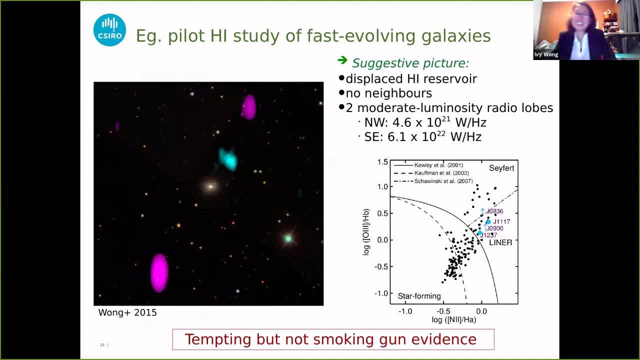 But yeah, we didn't, And we just ended up with this little puff of smoke at the same velocity. So so it's offset by about 70 kilometers per second. Okay, But given the size of the galaxy, this is well, well bound. 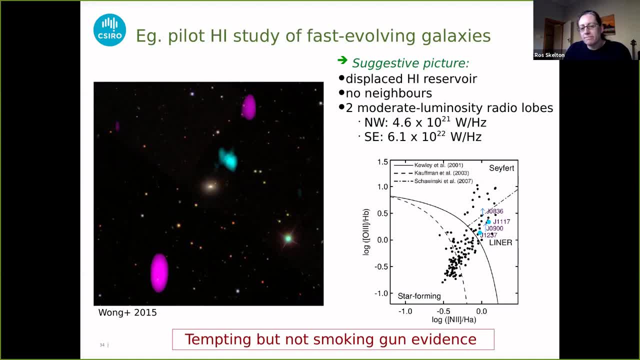 Yeah, very interesting. So this is actually a blue early-type galaxy And our pet theory is they're the predecessor population of post-starburst at the roughly the same redshift, And this is the most evolved of our four pilot galaxies, If you looked at the very, very young or the one at an earlier stage. 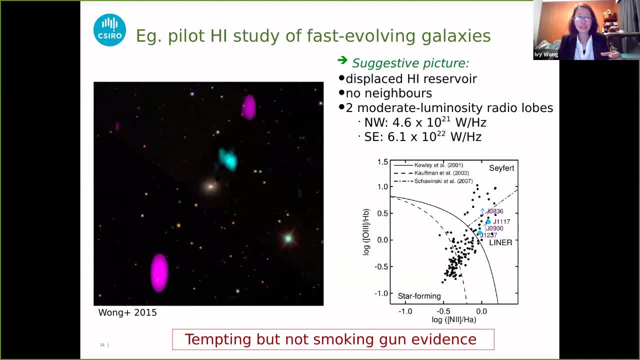 of evolution. the interesting thing is, the gas then becomes coincident with the stellar disk, but it's not rotating in the same direction as the stellar disk. So there's a fair bit of counter rotation, But once again we couldn't identify where the dwarf. 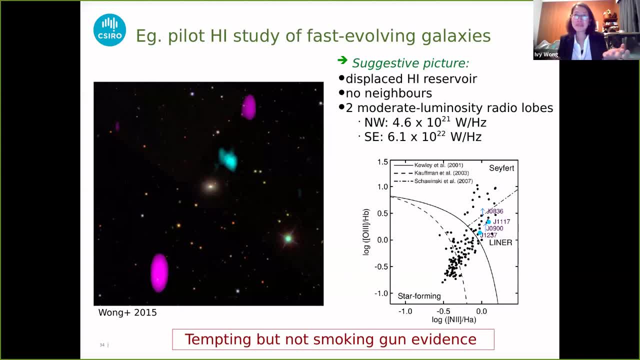 galaxy is, And these galaxies are not that far away. They're about six to 8,000 kilometers a second. So redshift of 0.025-ish, which is really nothing, or an optical sample, But interesting enough that we're not really sure what's happening. 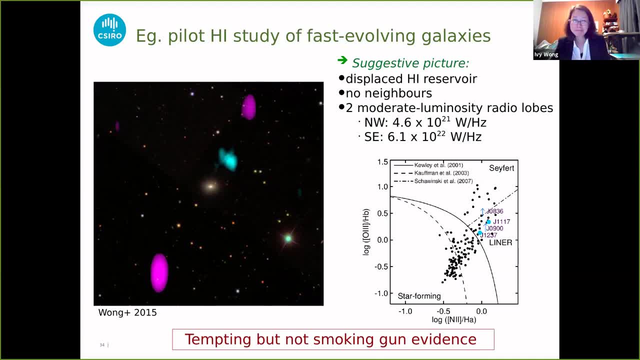 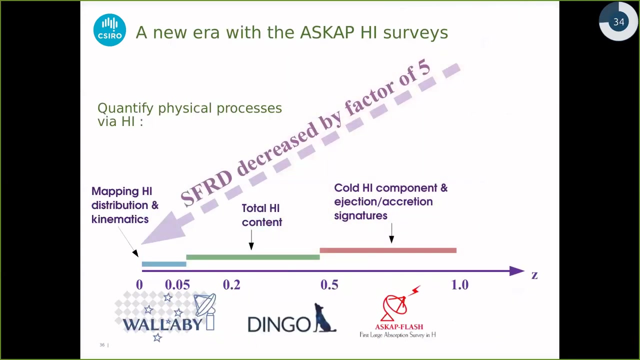 Thanks, No worries, Thanks for asking. Okay, Thanks, Ross. So there's a question from Shilpa Hi Ivy. Thanks for an interesting talk. I have a question about the early science wallaby observations of groups. Are there any planned observations of clusters? low range of clusters? 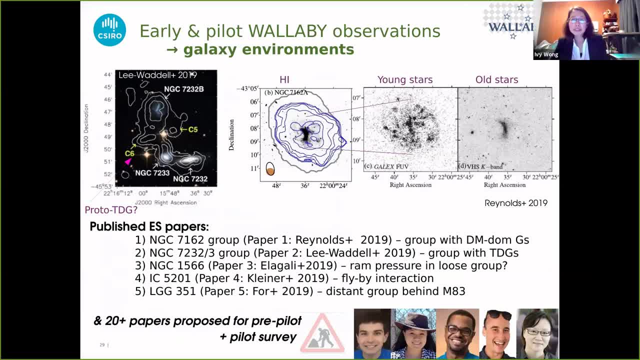 So the pilot observations have pointed itself at the Hydra cluster, So that's a main cluster. And there was a pre-pilot observation of the Eridana supergroup, which is sort of like a cluster, but it was only one of the subclusters, So it's a supergroup. 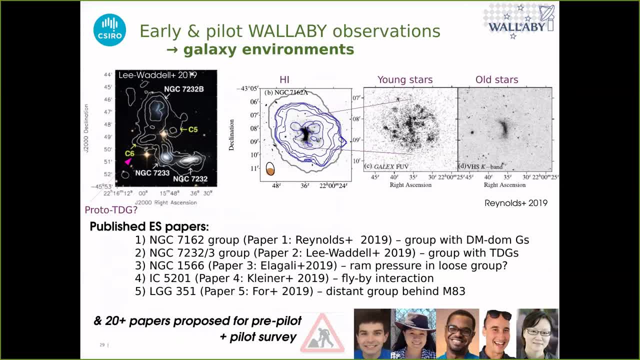 Thank you, No worries. Okay, Thank you, Shilpa. Is there any other questions Or any points that you need repeated, Because I have nothing better to I have a question about. I might not. Yeah, I don't know if this is a dumb question, but So. 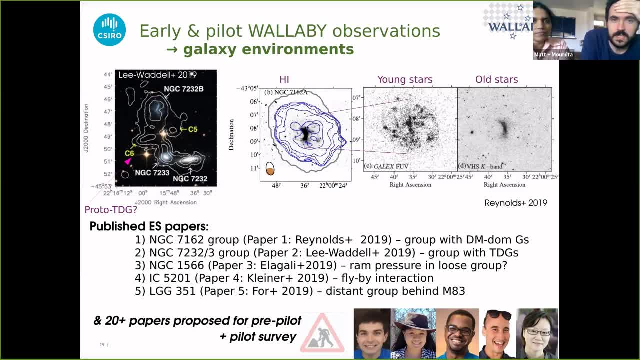 when you're talking about the CO and the ring galaxies, you mentioned dark CO. Ah, okay, I didn't quite follow what you meant by that. So dark CO is the CO that is colder and not emitting, So typically it resides in vestins diffuse environments, if that makes sense. 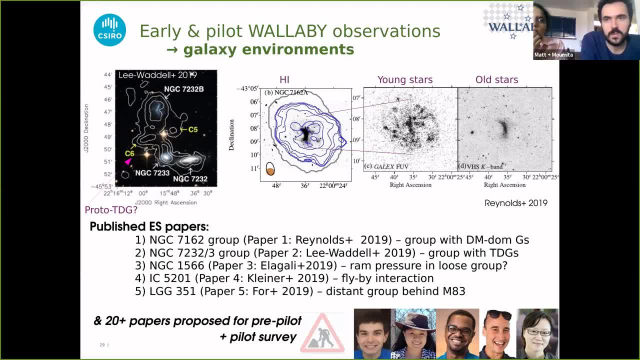 Okay, So it's just colder than the typical. The temperature of the CO1 gets detected- Oh, it's colder than what's required for it to a CO1 transition. Sorry, Okay, So is that just a denser gas or what's? It's just cold. 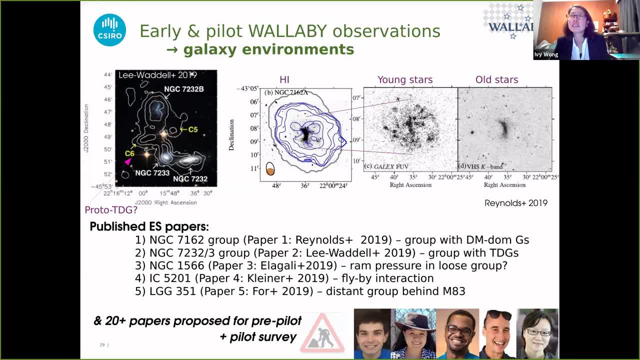 It's just colder. So the great thing is, at higher densities you're able to excite the gas to a A higher J transition state. Okay, So if it does get excited, and then we'll see the transition lines from one to zero. 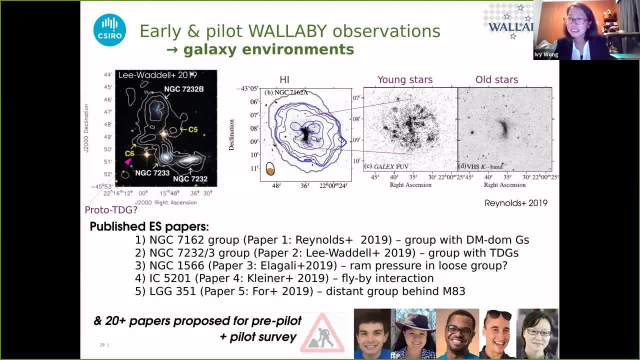 three to two, two to one: Okay, If nothing happens to it then it just hangs around. But given how exciting the ISM of a ring galaxy is, it is unlikely. Okay, Thanks, And the bizarre thing is all the CO we found in the ring galaxy. 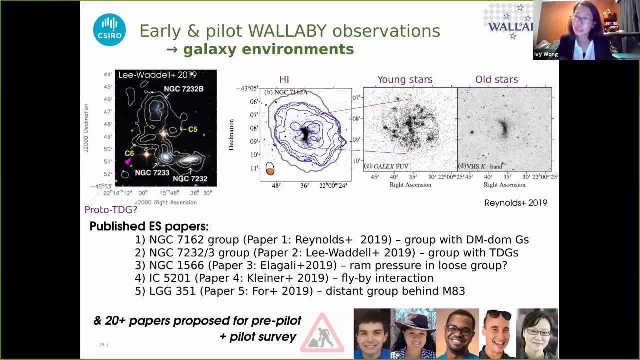 actually is in the bulge in the core regions, not in the ring. So I think the ring really does destroy the molecular gas very fast through the giant bursts of star formation. And the interesting thing is that there are a lot of ULXs, so ultra-luminous X-ray sources, embedded within rings of ring galaxies. 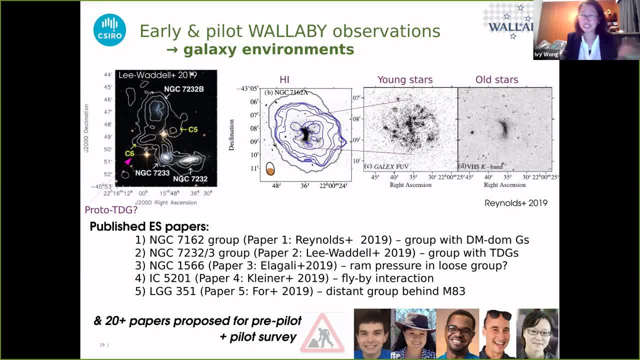 Okay, Thanks. So the initial mass function is also different. Okay, Thanks. So in case you're interested in star formation and initial mass functions, it throws everything we know out the window, essentially. Okay, Claude, you have a question. Sorry, go ahead. 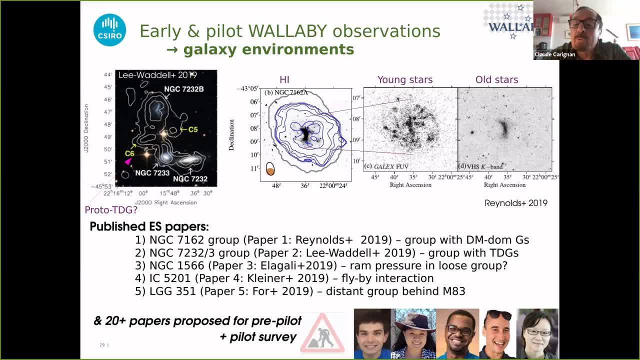 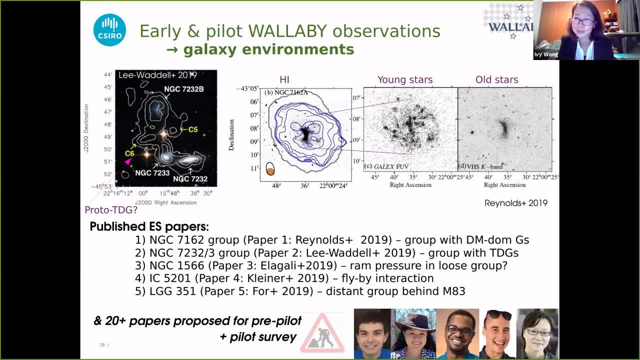 They're trying to get it reduced a second time because we had so many. Well, we had quite a fair bit of trouble getting a clean map or a clean cube out of it, But I think that we've sorted out quite a few of the issues. 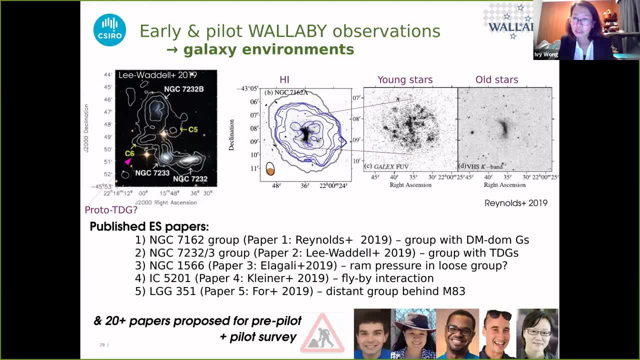 And so DR2 should be. So data release 2 should be imminent for Hydra. Okay. The other two fields will have to wait a bit longer because some of the other surveys are taking up the computing time. Okay, but we're talking about a few months to get the data out of that field for that Hydra field. 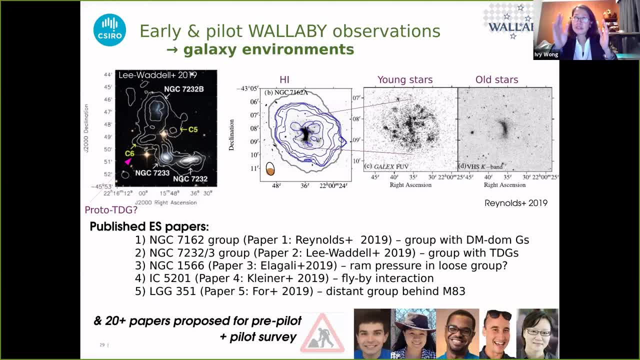 So the data is already out. if So, some of the data's already out. Yeah, So there's been a release of a sub region. I can actually email you the link to that particular. Okay, Are you interested? Yes, Yes. 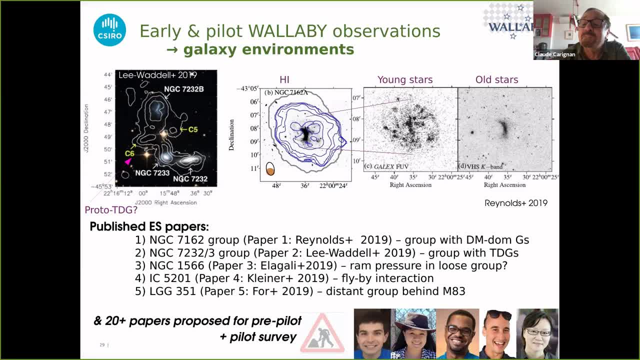 Thanks a lot. If you can email that, that would be great. Cool Will do. Thank you, Actually write it down so I don't forget.